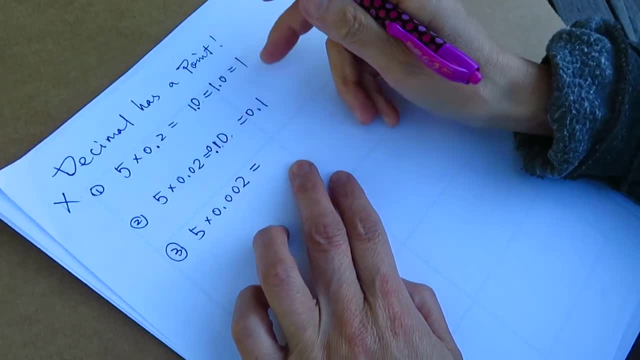 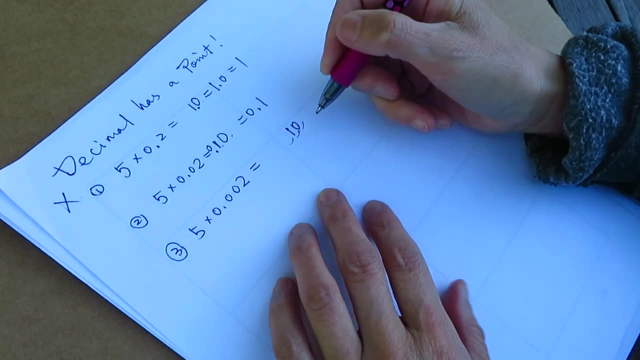 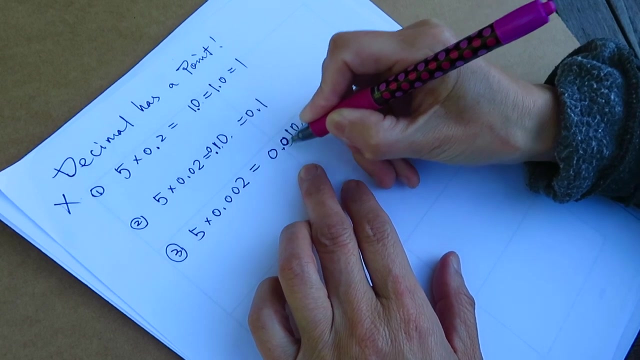 And this one. you can just keep on repeating three zeros: 10,, 1,, 2, 3.. And another thing I let my students know is 1,, 2, 3.. So it's 0.01.. 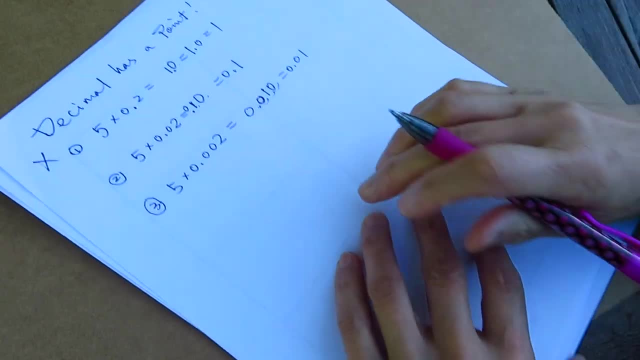 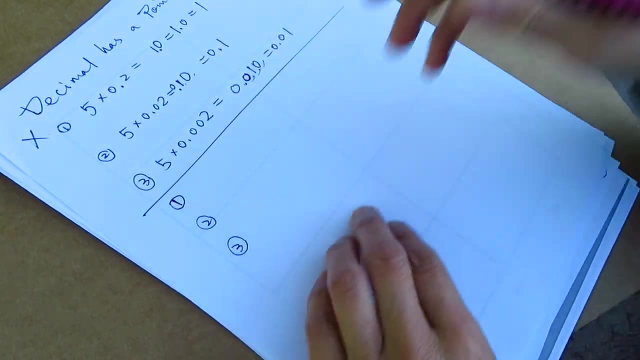 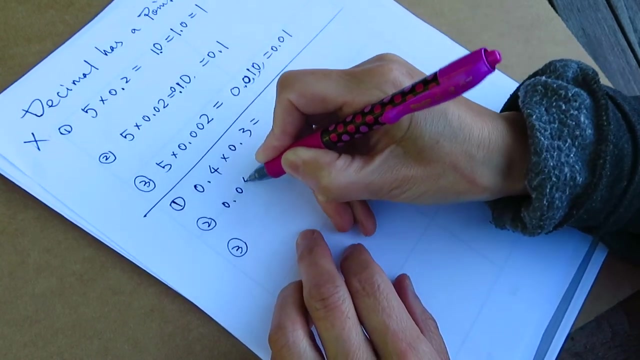 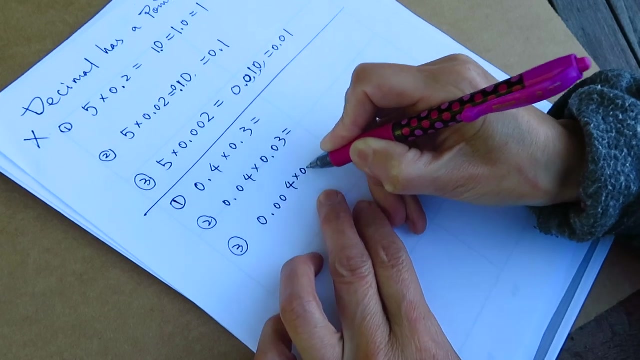 0.01.. Do I make sense? I write it even larger. Now we do another three: 1,, 2, 3.. So this one 0.4 times 0.3.. 0.04 times 0.03.. 0.004 times 0.003.. Those so many zeros. 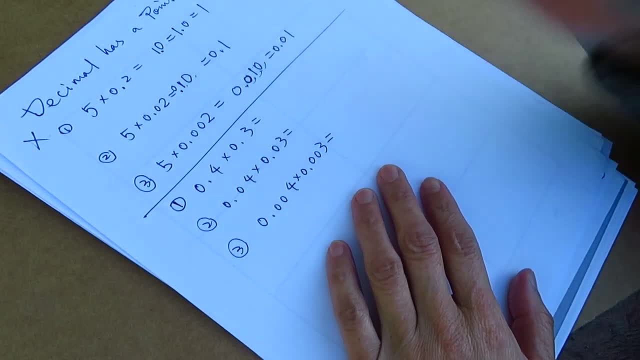 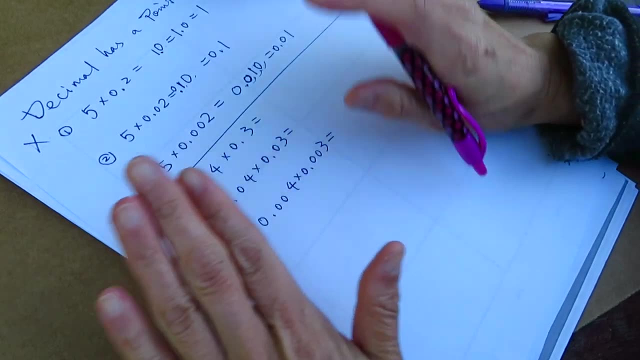 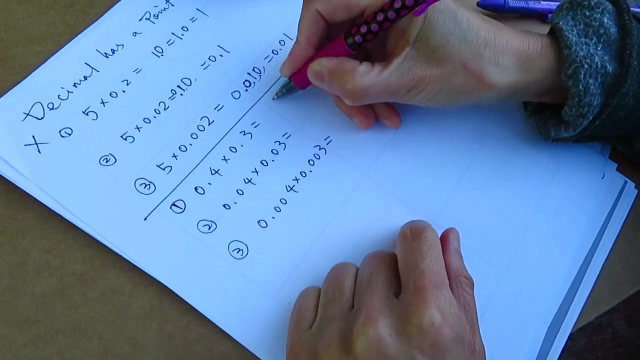 Looks so complicated, right? What do we do? Let me get a pencil, Let's continue. So I tell students one of the things. First, forget about decimals. You do only the number calculation: 3 times 4.. 4 times 3 is 12.. 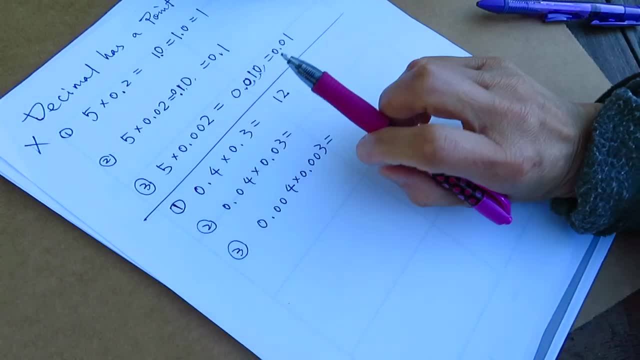 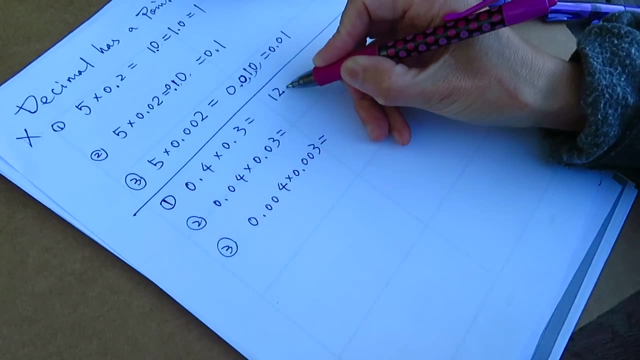 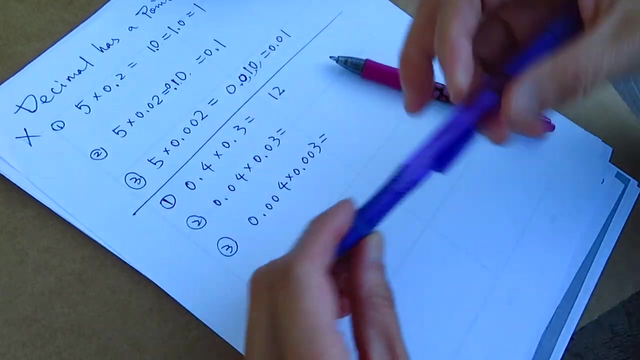 And then you count how many numbers behind the decimal, How many points 1, 2.. Two numbers And you need to move your decimal, point 1, 2.. Uh-oh, If there are many you will forget, right. So let's see This one we will move. 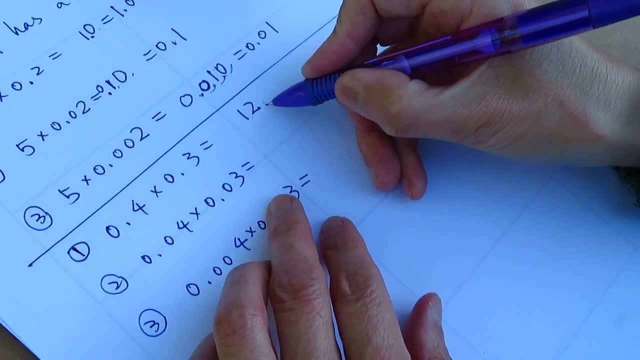 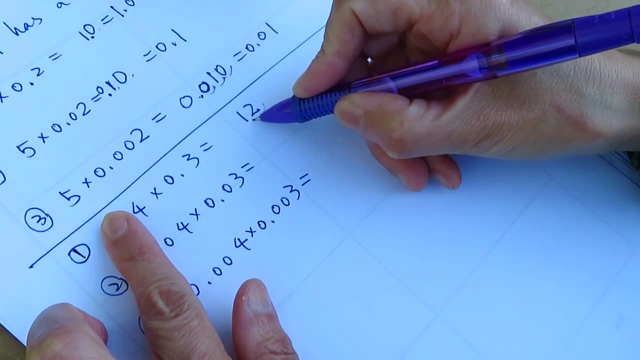 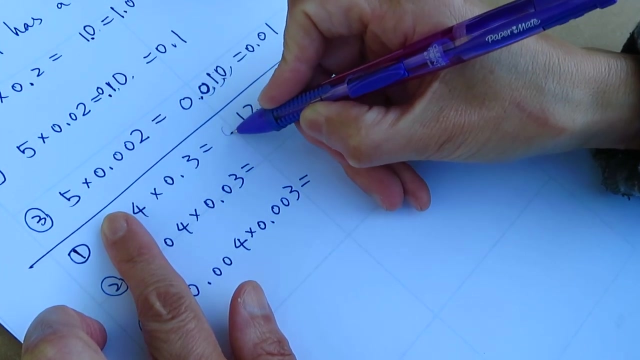 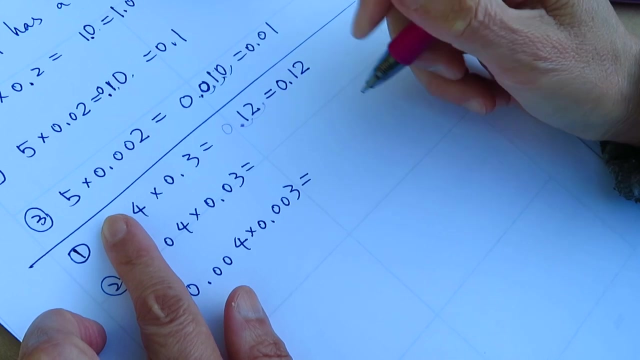 Originally the decimal point here is here right. Here is 4 times 3 is 12.. 1, 2.. So it's here. You move 1, 2.. Two points add a zero here, So the result is 0.12.. And this one so many decimal points, it becomes complicated. 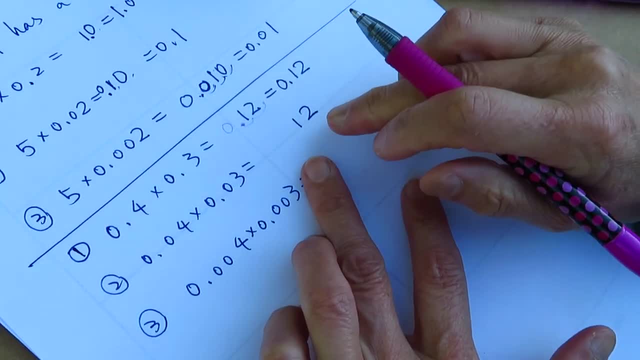 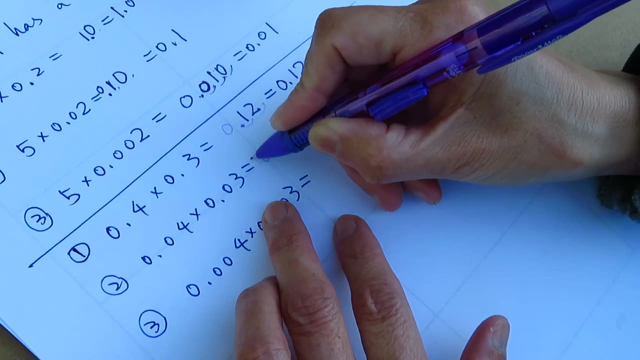 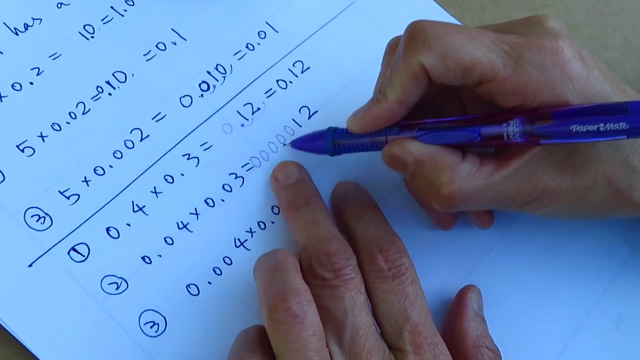 and easy to forget. what do I do? you write down the final result number and put a lot of zero ahead: one, two, three, four, five, six, seven. put many decimal points, because anything behind zero, behind the real number, it does not count. it's still 12. I didn't. 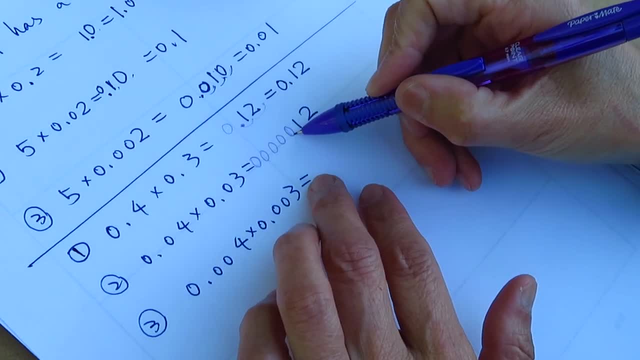 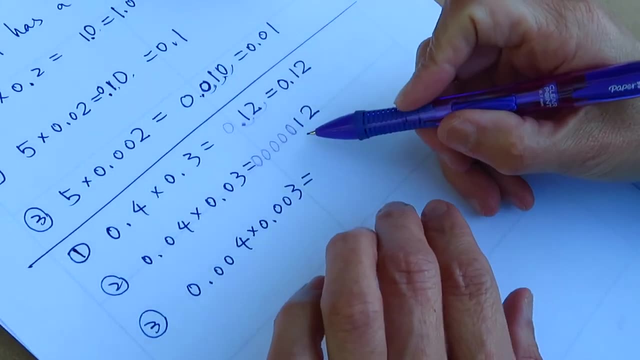 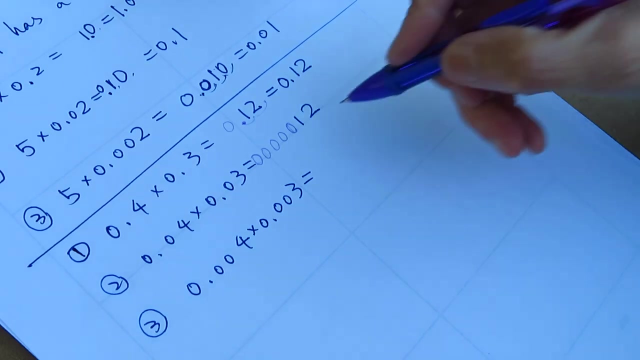 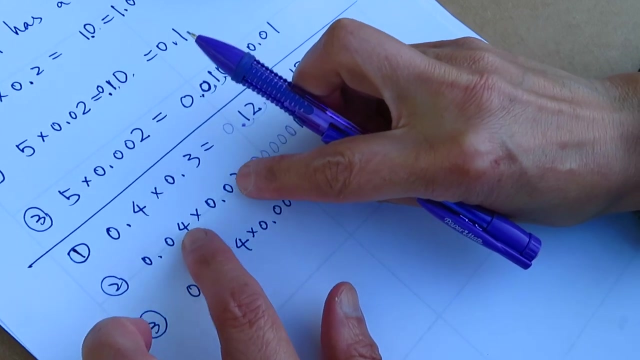 change any value because behind in front of the number I add many zeros. it does not count or it's. the value is 0. you did not change any of the real value of this 12. now one, two, three, four, four places behind the decimal, so I need to move the. 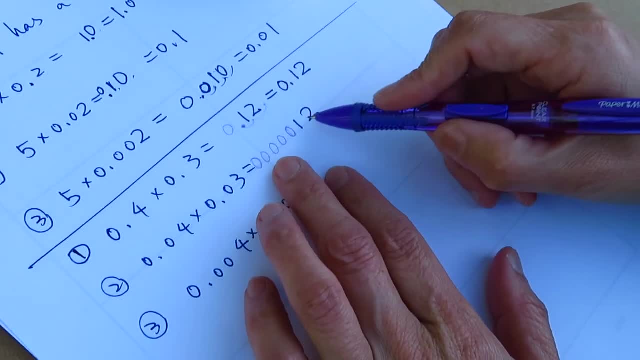 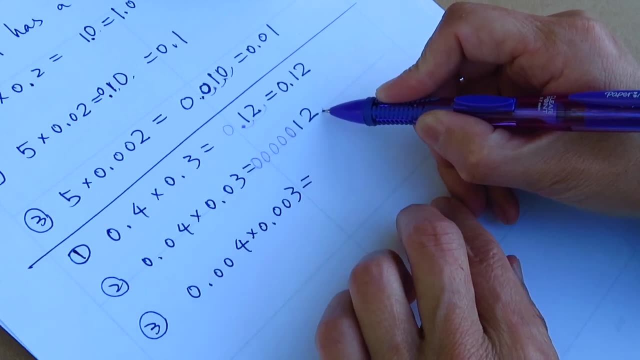 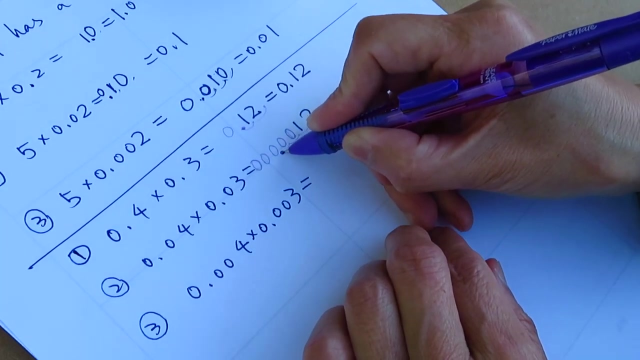 decimal point 4 places. so I put this so that I'm easily to move the decimal point. originally it is here: 1, 2, 3, 4, Tatang. I stay here. so this is the number I need to write down and before it it does: 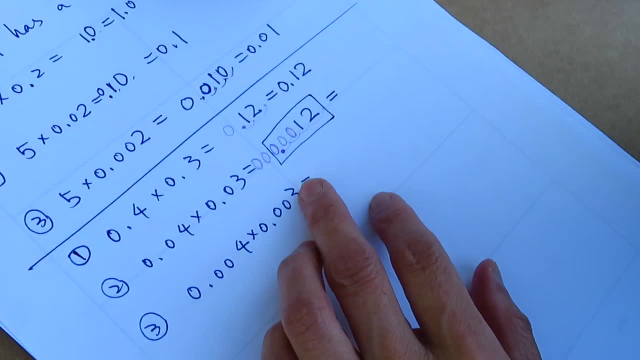 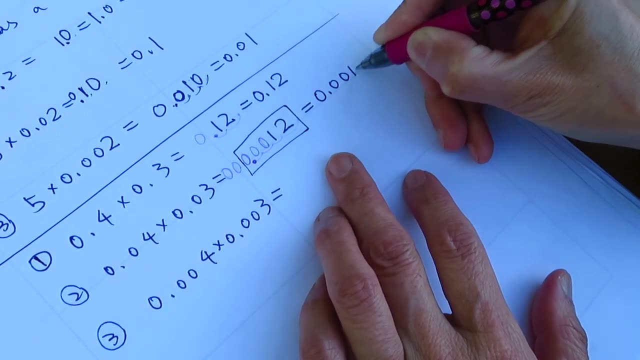 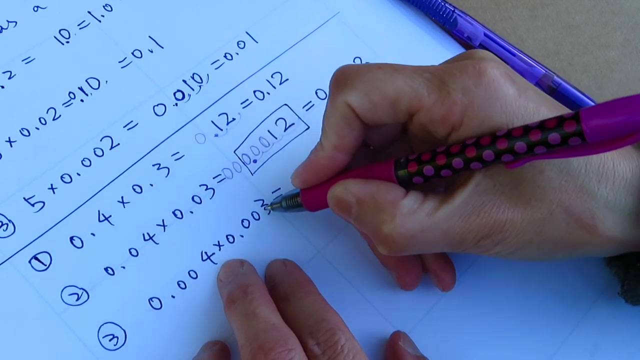 not count. it is not good for this, for these, this little trick. So 0.0012.. 1, 2.. Okay, the same thing here. We get 3 times 4, 4 times 3 is 12.. 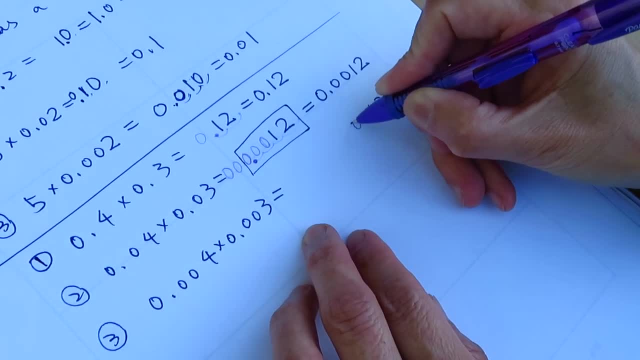 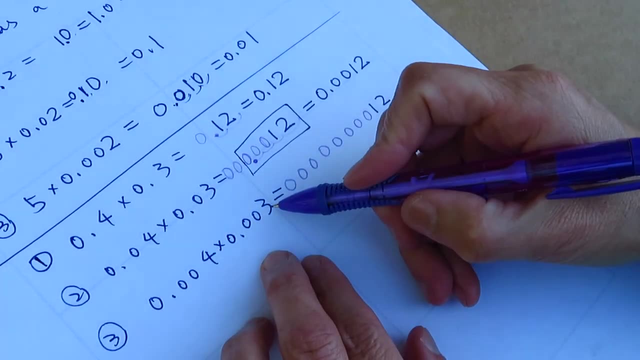 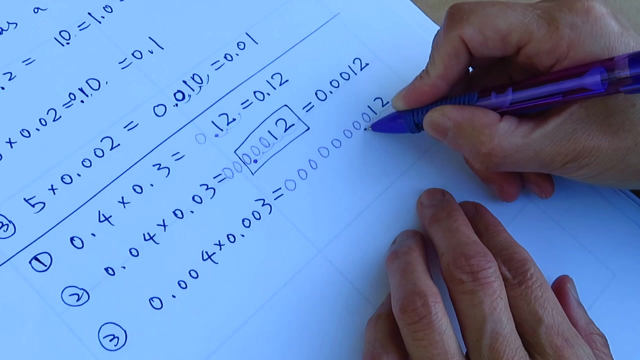 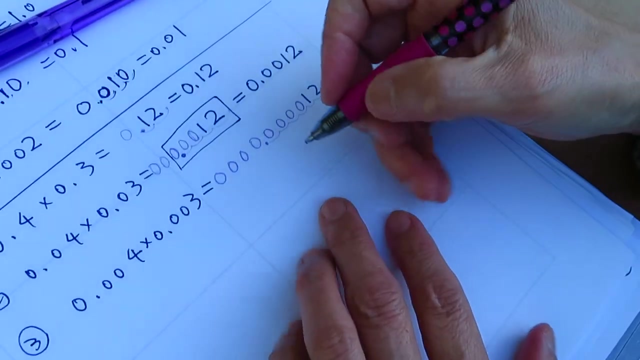 Oh, so many decimal points. Let me just keep on writing the zeros. Keep on writing many, many zeros: 1, 2,, 3,, 4,, 5, 6.. Here: 1,, 2, 3,, 4, 5, 6.. Stop, Okay, now we get the number we want. 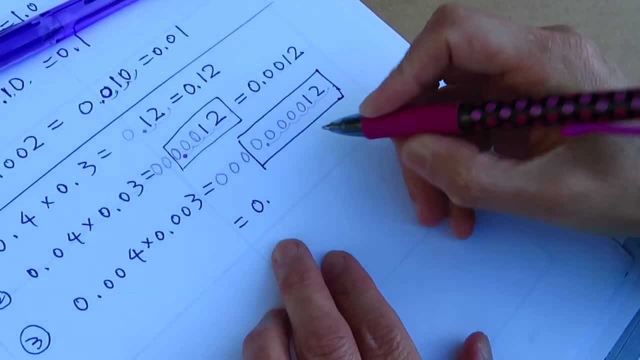 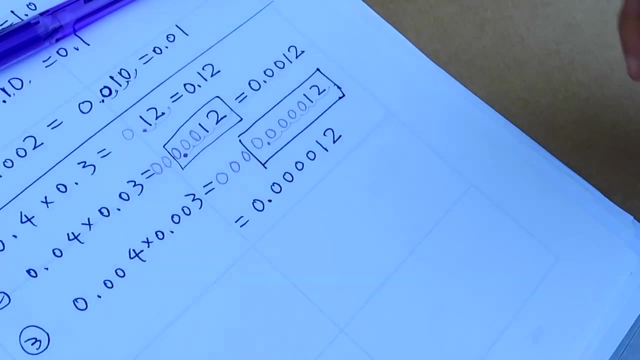 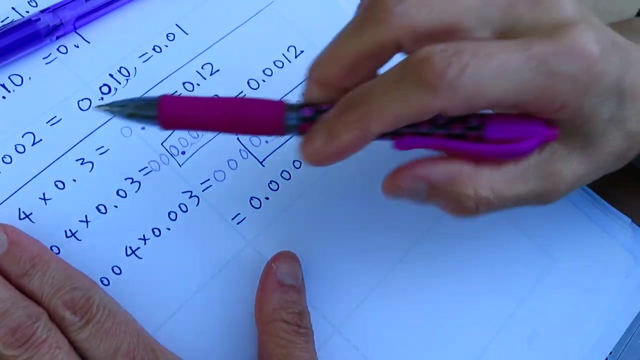 So it's 0.1234.. 0, 0, 0, 0, 1, 2.. Is that easy, Easy peasy, lemon squeezy, isn't it? Just remember when you do forget about the decimals. 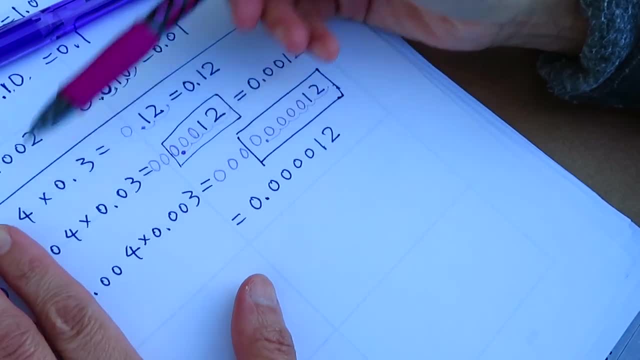 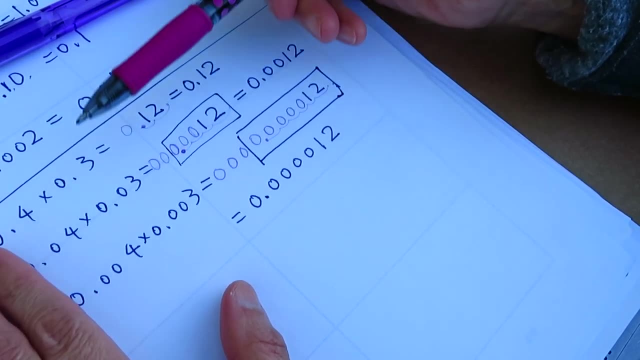 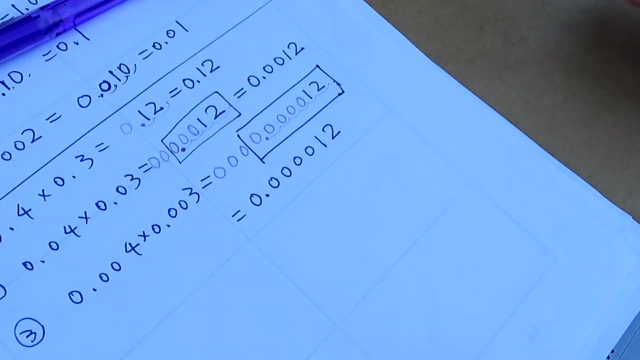 Do the real number, real number multiplication. Later we will do division- It is the same thing, Real number multiplication- and then count the decimal points. How many places behind the decimal points? Okay, now this one, we will do a little bit complicated. 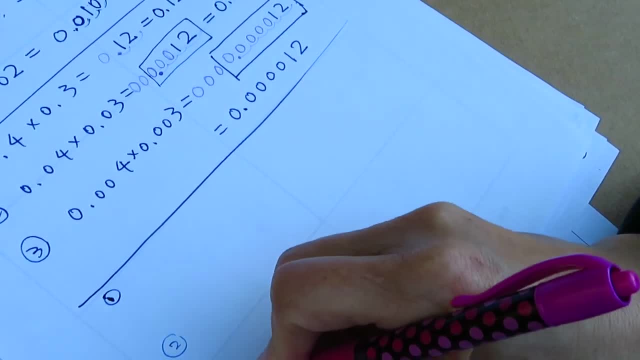 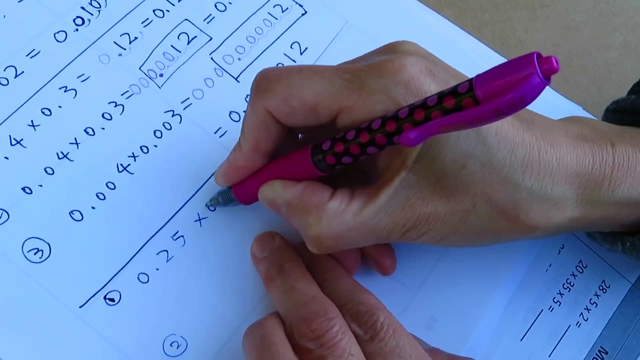 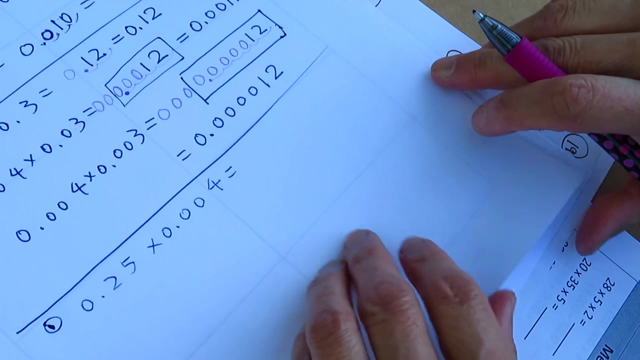 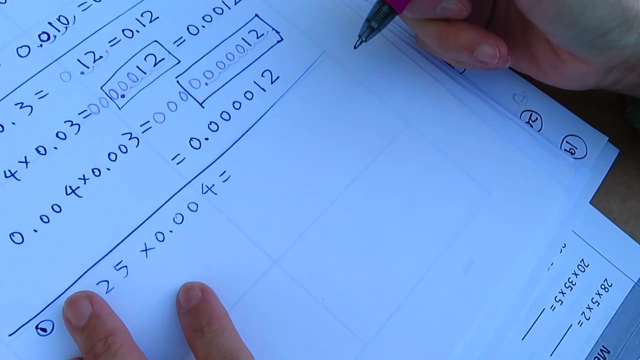 Number 1,, 2, 3.. 0.25 times 0.004.. Okay, So now we will do 1 at a time. We know 25 points times 4 is 100, right, Because a quarter is 25 cents. 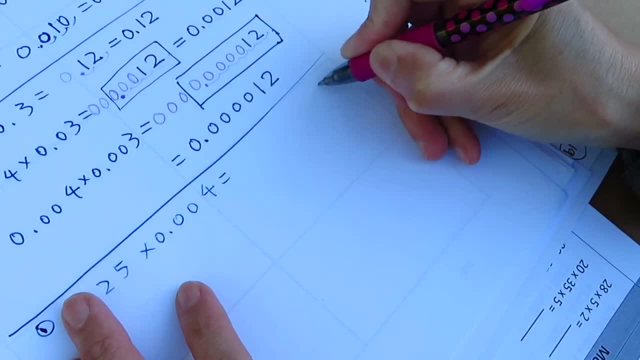 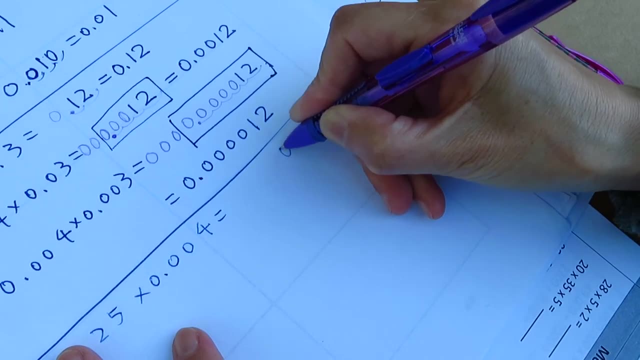 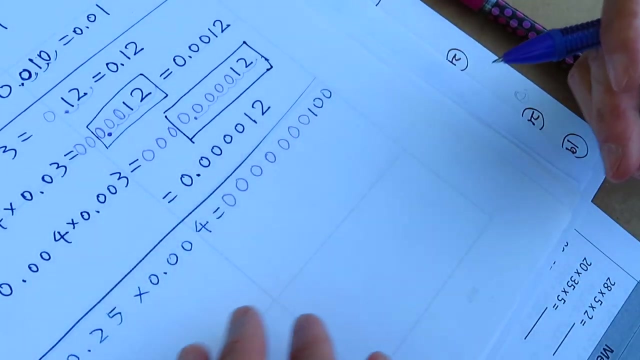 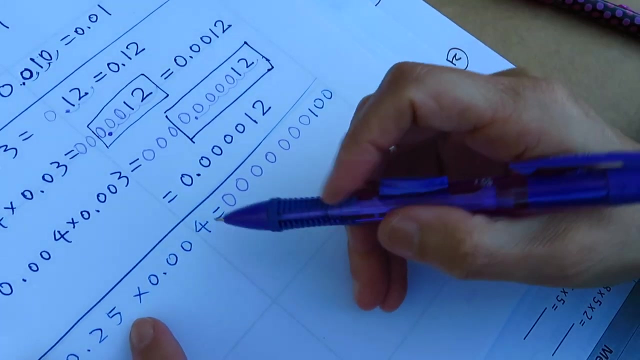 quarters. we make one dollar, right, so 100. we write it down and put zero behind in the front. just put a lot of zero. i mean you do not need to put really a gazillion zero, you know, because the total is four or five or six. six is sufficient enough, okay, one, two, three, four, five. 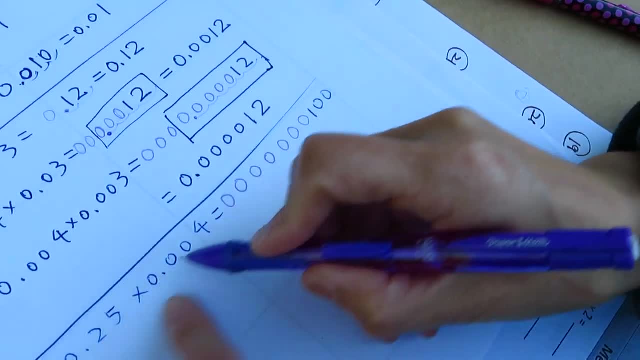 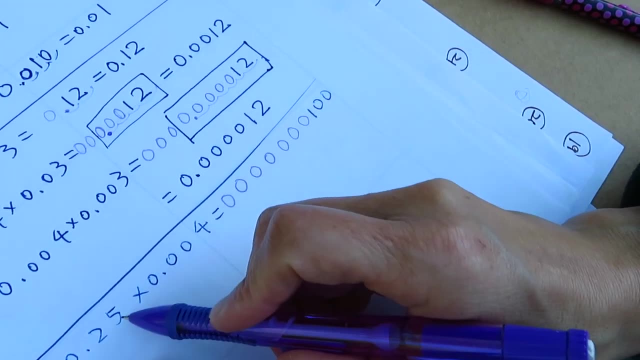 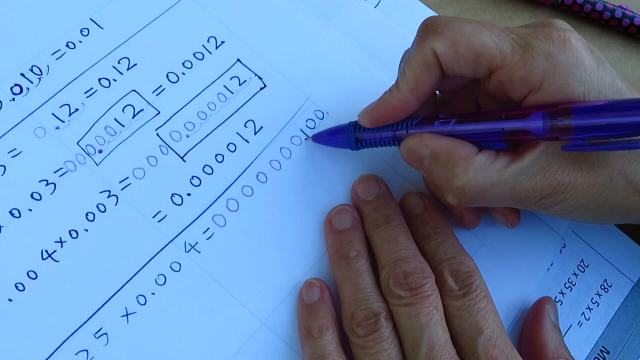 five, we need to move for five points. 25 times four is 100, so we get the, the, the 100 written here. one, two, three, four, five. starting from here, one, didi, two, didi, three, didi four, didi, five, five. one, two, three, four, five. starting from here: one didi two, didi three, didi four, didi five. 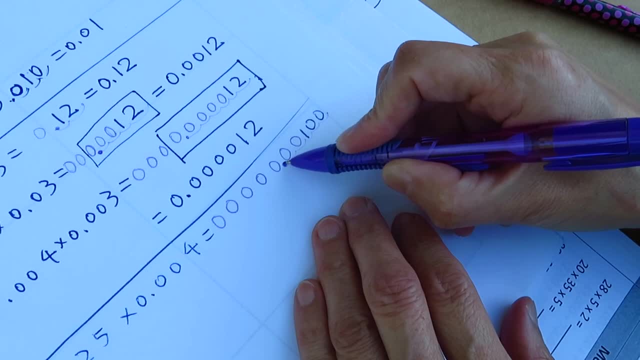 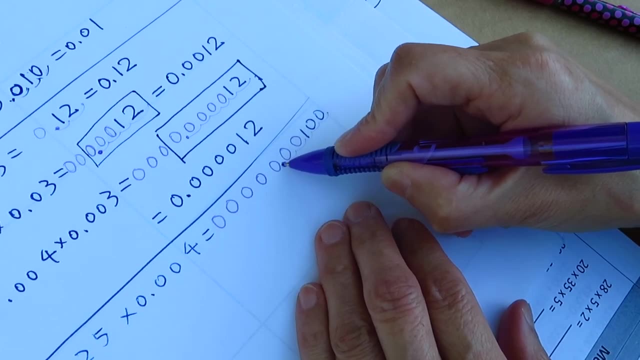 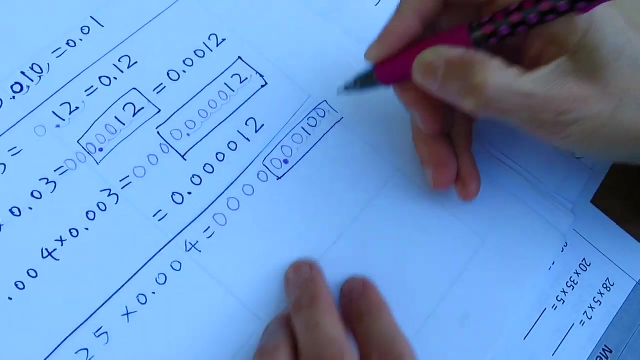 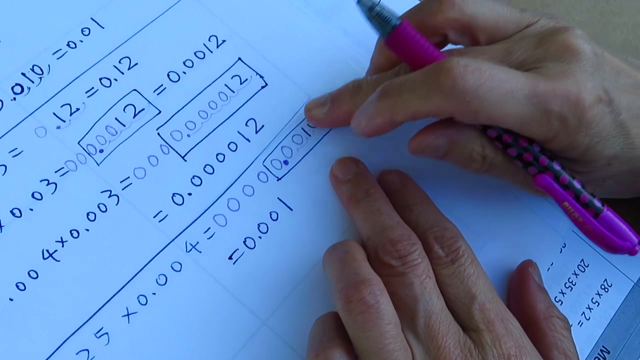 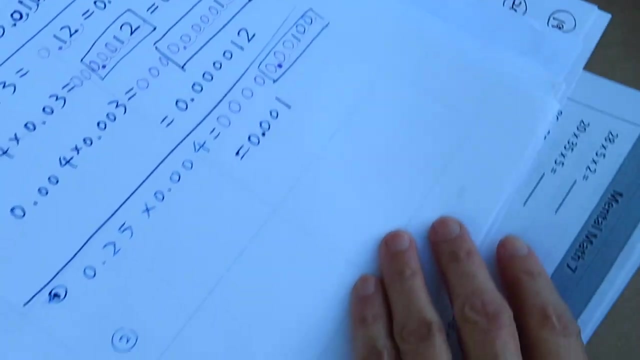 5.. Okay, we will stop Station here. It's like a ship: I am sailing, I am sailing. Okay, stop Until 5, we stop Equals 0.001.. Okay, these two zeros. you do not need to write it, But so that you can remember how you do the calculation. 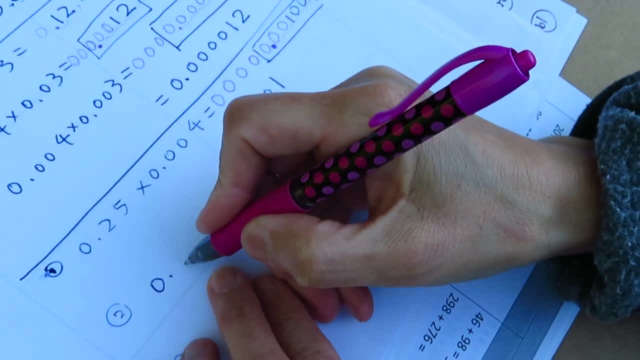 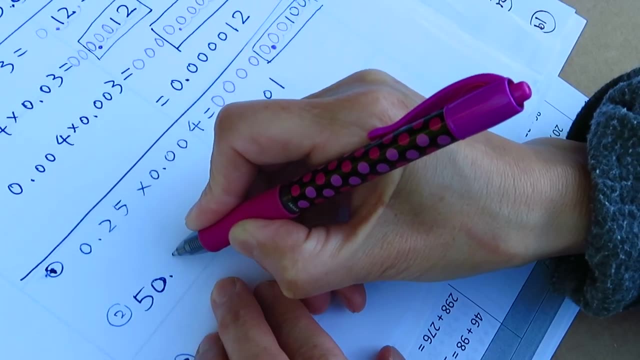 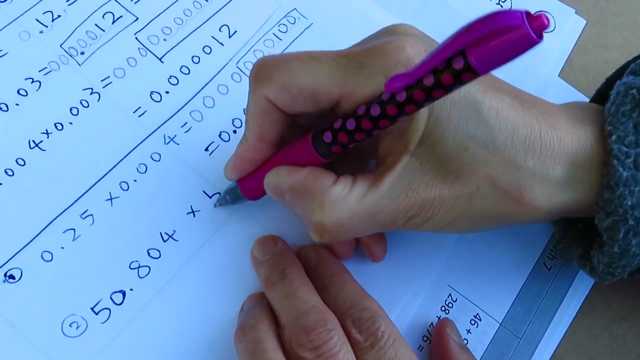 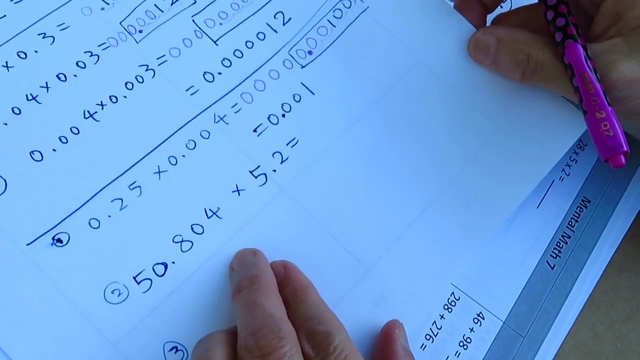 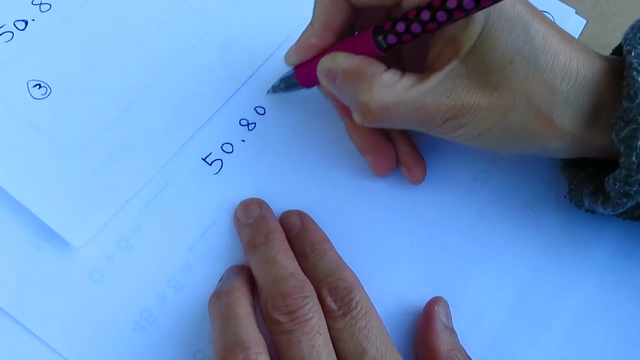 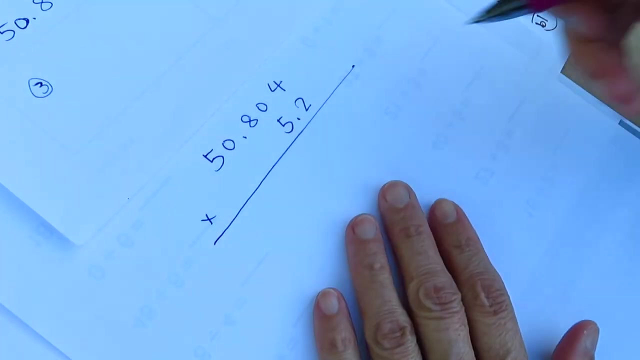 This one, we will do 0.50.7804.. Times 5.2.. Okay, let's do it. This one is a real calculation. We will do it 5 times 5.82.. And do the calculation. There is not much trick, You just honestly do it. 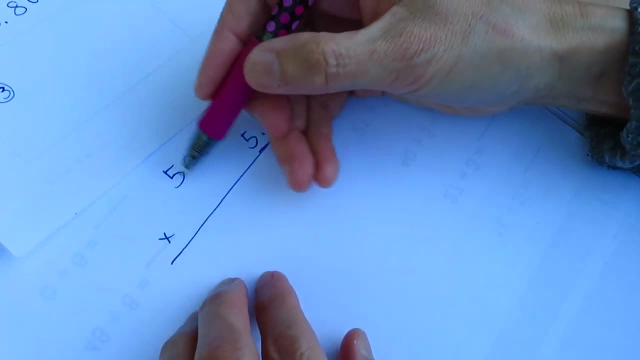 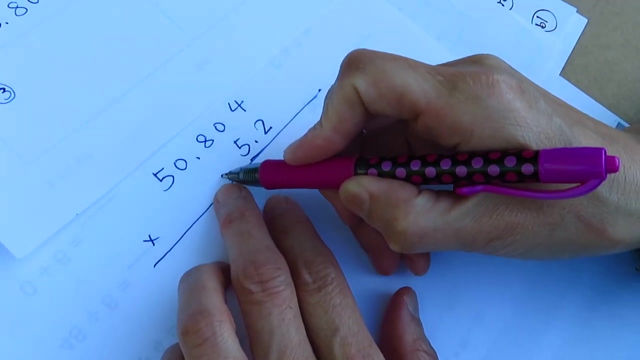 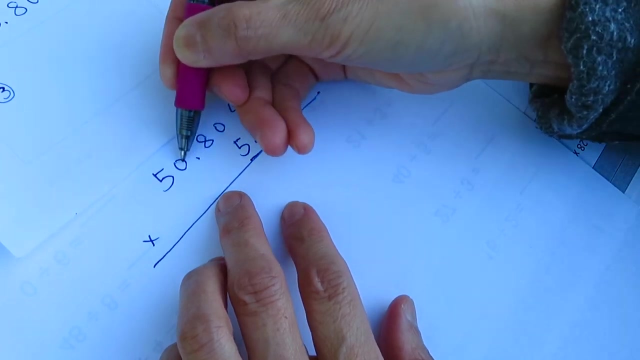 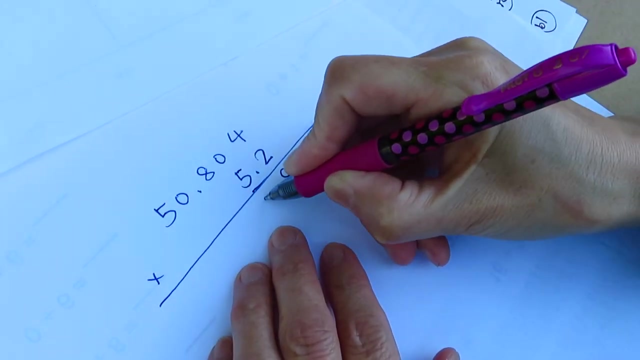 Each line goes with each line. Make sure the place value is correct And you do not need to place the decimal point with this In multiplication. make sure all these numbers, one by one line together: Okay, 2, 4, 8, 0, 2, 8, 1, 16,, 2, 5,, 1, 16.. 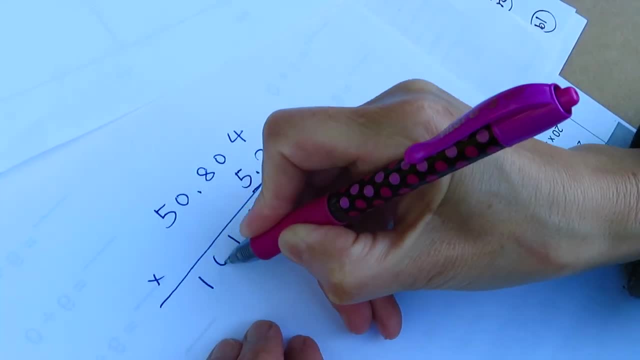 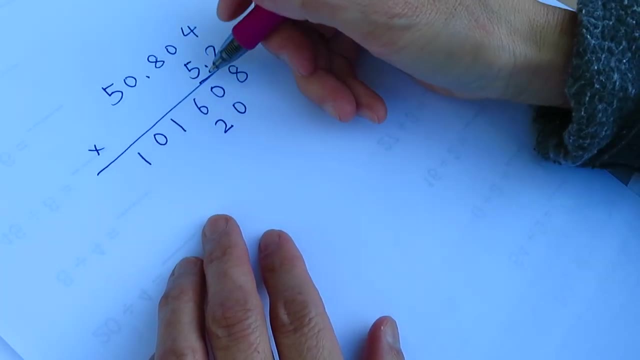 2, 4, 8, 0,, 2, 8,, 1, 16,, 2, 5,, 1, 16.. 1, 10.. Okay, make enough room. 4,, 5,, 2,, 10.. And this place is 0.. I have a habit: I do not write it down. 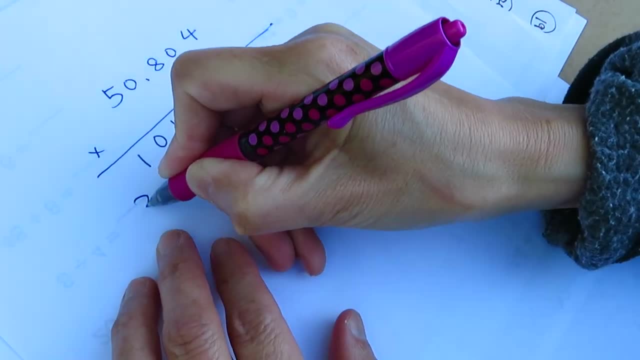 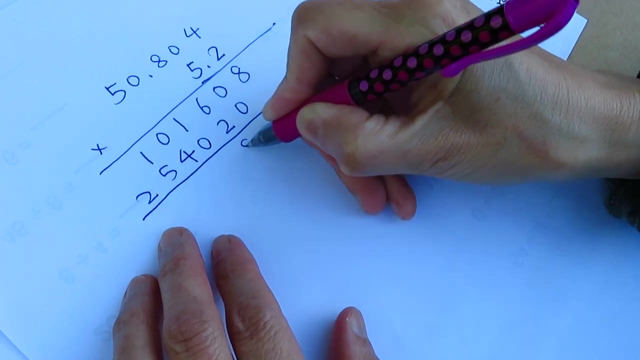 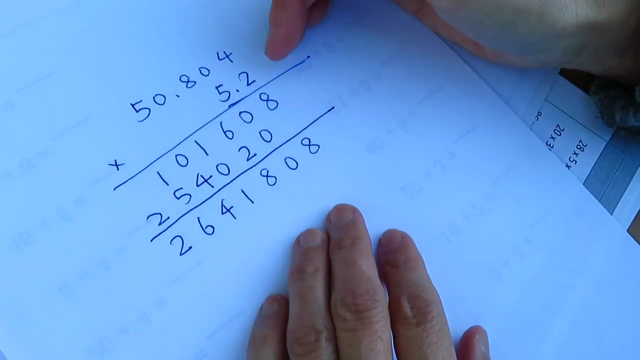 5,, 8,, 4,, 10.. 5,, 5,, 2, 15.. So we first do the real calculation: 0,, 8,, 1,, 4,, 6, 2.. Okay now, after we finish doing the calculation, 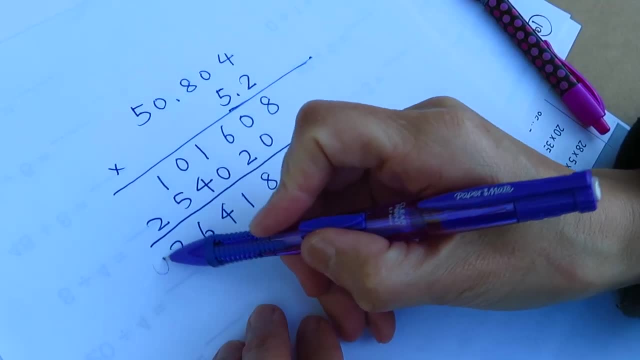 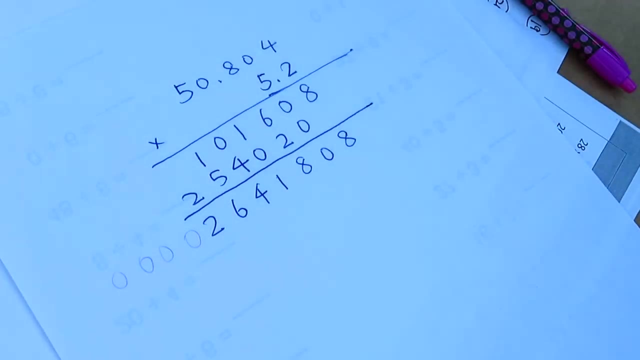 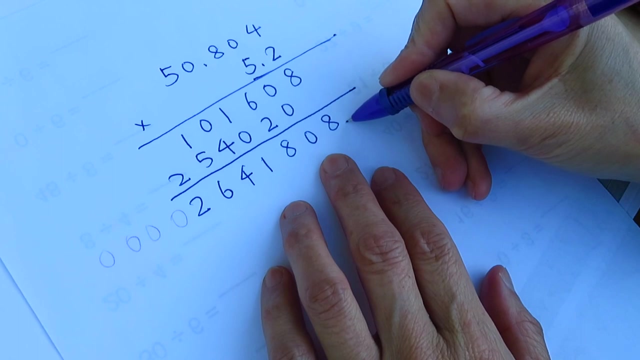 what we need to do. we need to count zeros In front of it. you can add 0 or not to add 0. That is not so For now. we do not need it. 1, 2, 3, 4.. Four decimal points. 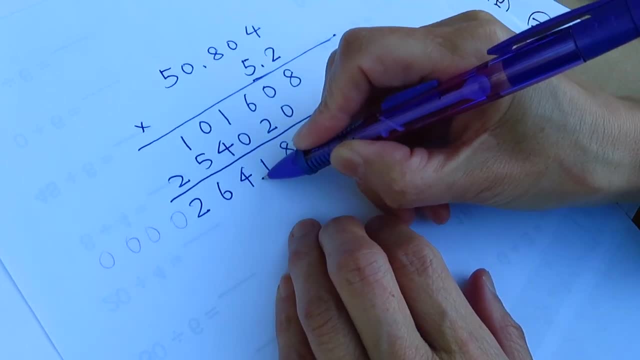 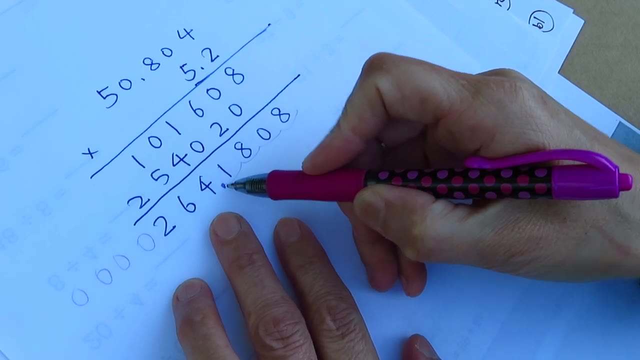 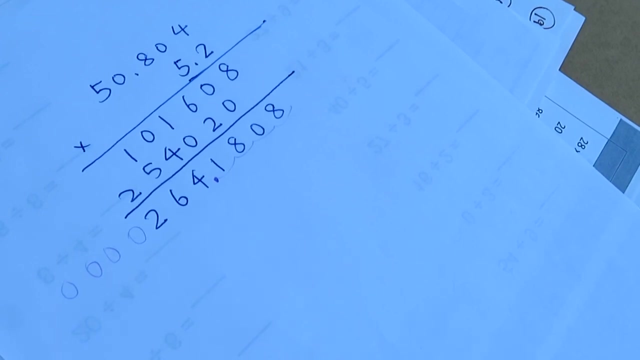 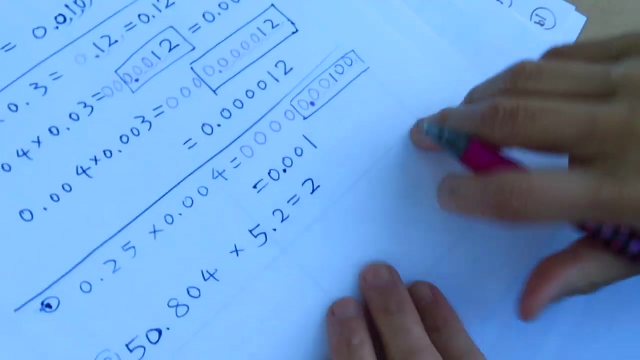 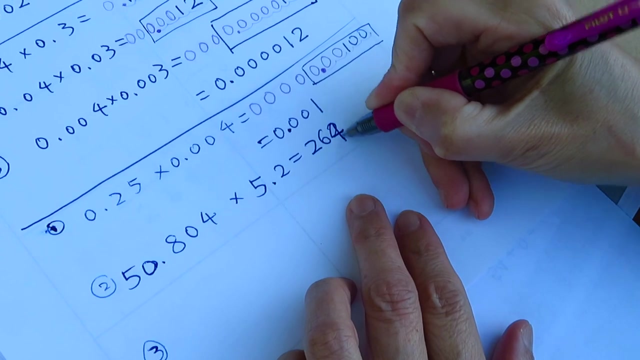 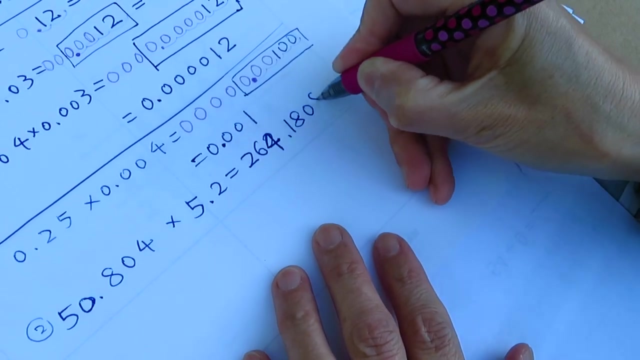 1,, 2,, 3, 4.. Okay, stay here. So the value is 264.1810.. Oh, 180.. Let me get it down a little bit, So that is 264.1808.. 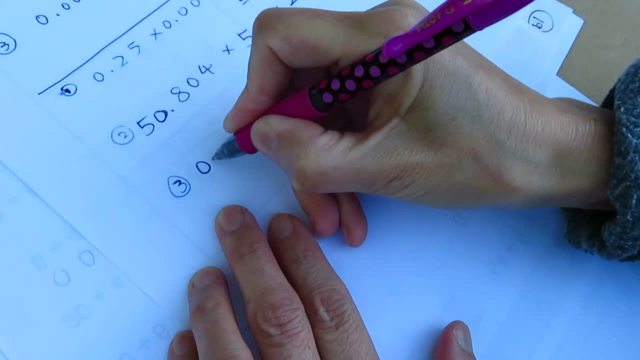 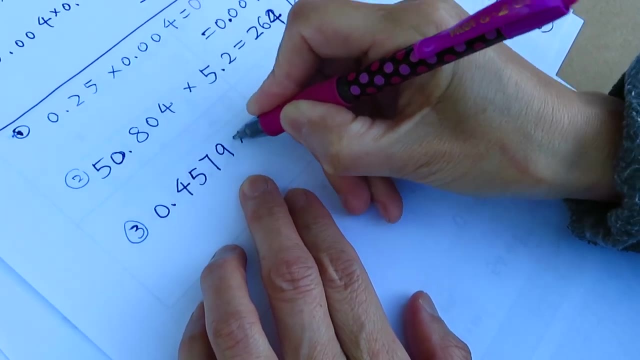 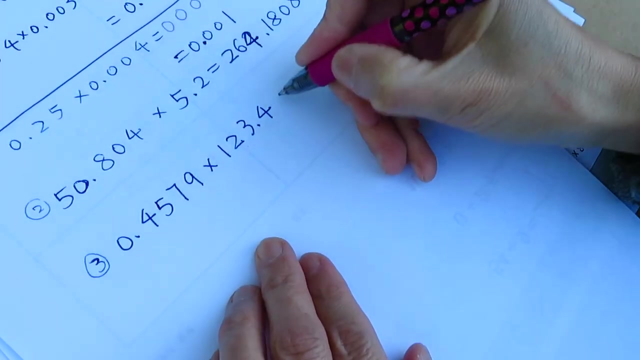 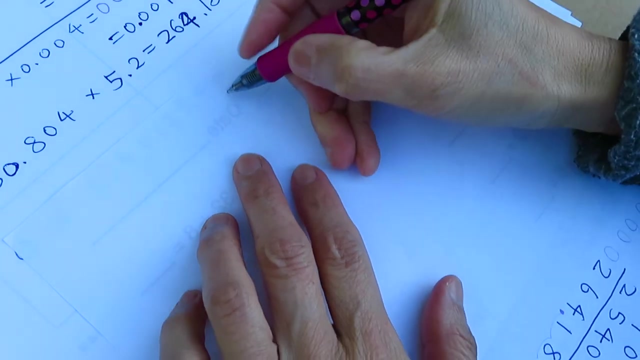 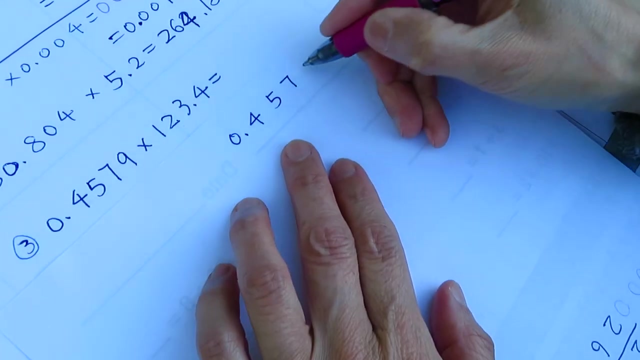 Now this one, we will do an even bigger one: 0.4579 times 123.4.. I like this. Okay, let's do it. Write it here: 0.4579.. 7, 9.. Times. 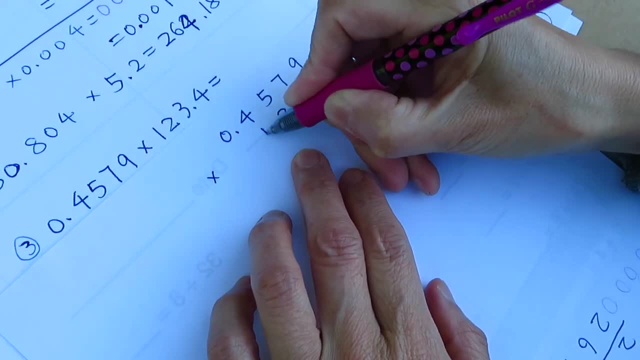 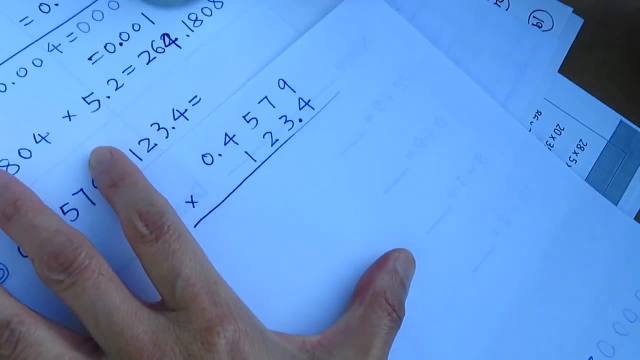 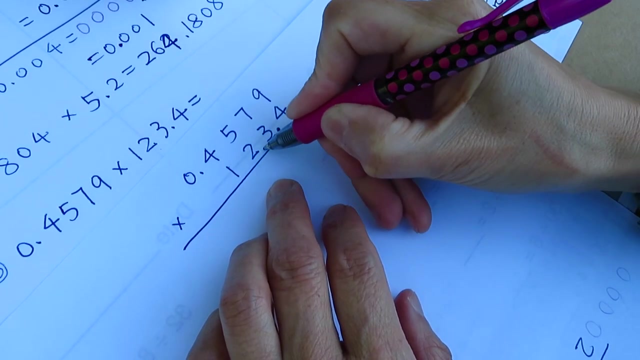 4,, 3,, 2, 1. Make sure There is no point 49.. 36. 47,, 28.. 28, plus 3. 31. 45,, 20. 23.. 41,, 16. 1,, 18. 39,, 27. 37,, 21. 23. 35,, 15. 1,, 17. 34,, 12. 1,, 13.. 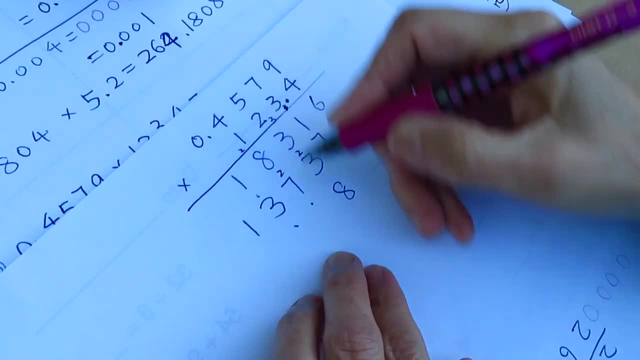 29. 1,, 10. 1,, 18. 27, 1,, 14. 1,, 15. 25,, 1,, 10. 1,, 11. 24,, 8.. 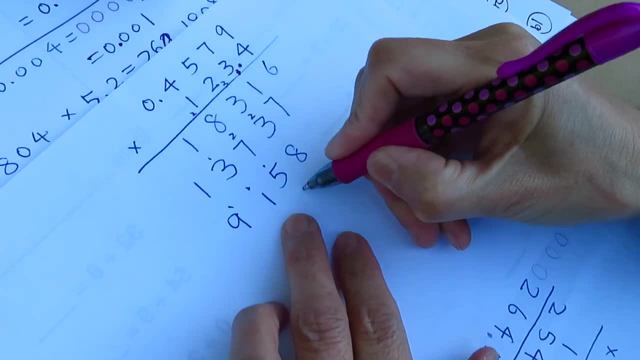 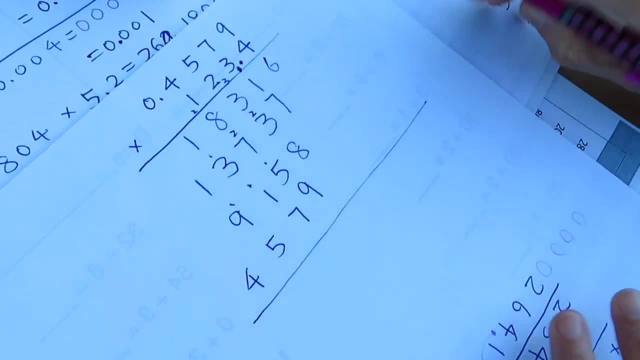 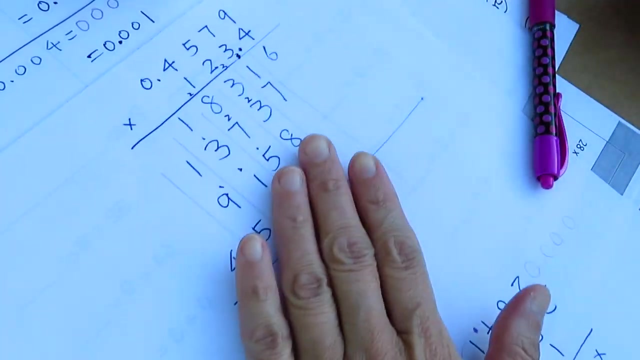 Plus 1,, 9. 15,, 9. 17,, 7. 15,, 5., 14,, 4.. See our line. Even without the ruler, we leave enough room for us to write it down. 6,, 1,, 7,, 8.. 6, plus 8., 14., 15,, 20., 20, plus 10., 30., 30., 70., 10., 11., 12.. 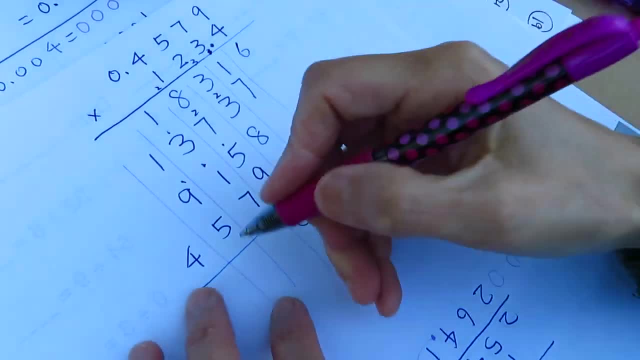 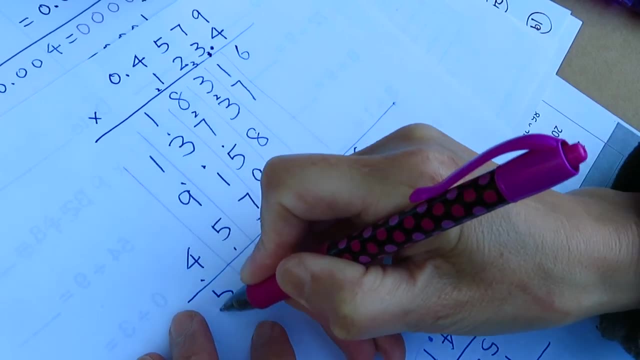 15. 16.. Okay, So we will first do the real calculation. After that we will count how many decimal points we have: 1,, 2,, 3,, 4,, 5,, 6,, 7,, 8,, 9,, 10,, 11,, 12,, 13,, 14,, 15,, 16,, 17,, 18,, 19,, 20,, 21,, 22,, 23,, 24,. 24,, 25,, 26,, 27,, 28,, 29,, 30,, 31,, 32,, 33,, 34,, 35,, 36,, 37,, 38,, 38,, 39,, 40,, 41,, 42,, 43,. 41,, 42,, 42,, 43,, 44,, 44,, 45,, 45,, 46,, 47,, 48,, 49,, 41,, 42,, 45,, 46,, 47,, 48,, 49,. 40,, 42,, 44,, 45,, 47,, 49,, 40,, 44,, 45,, 48,, 50,, 51,, 42,, 42,, 44,, 45.. 1,. 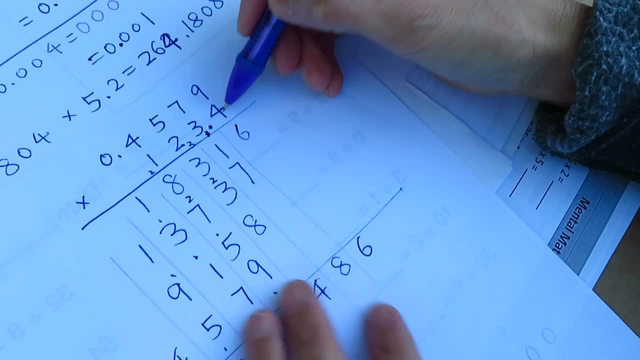 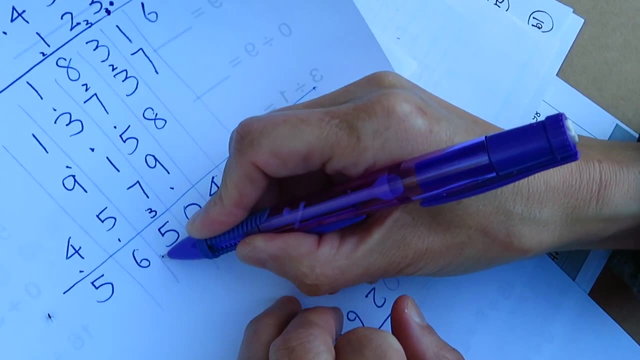 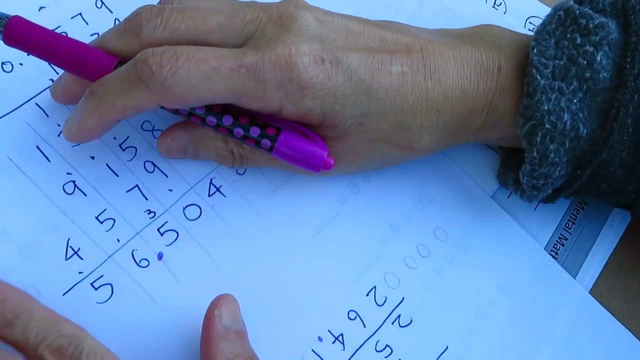 2,, 3,, 3, 4, 5.. Okay: 1, 2,, 3,, 4, 5.. Stay here. Stay here, Okay. So the result: the result is 56.50486.. 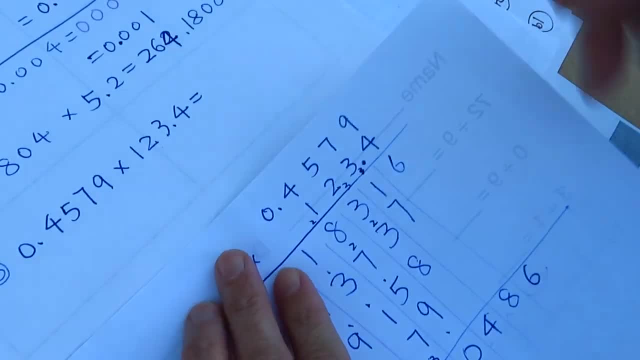 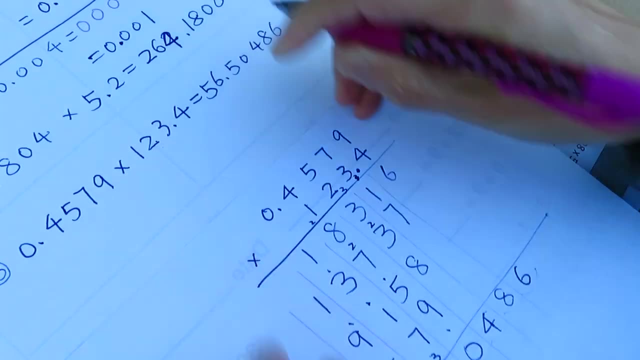 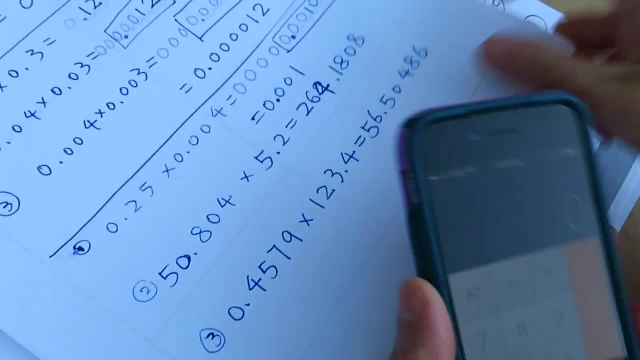 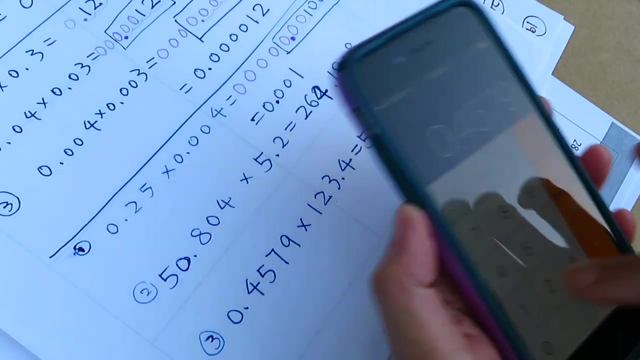 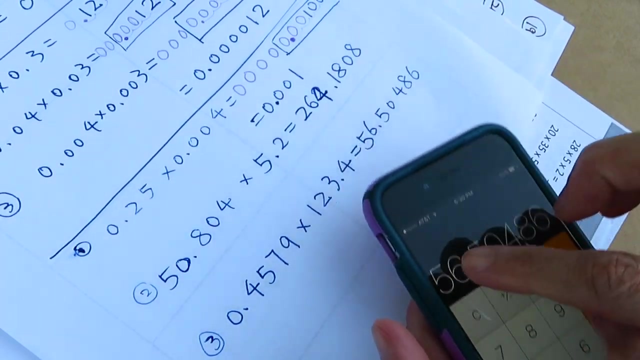 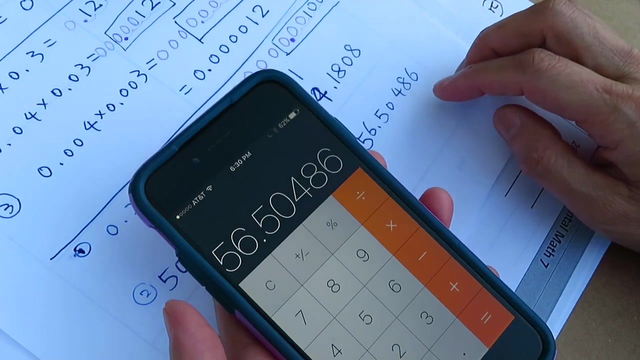 Congratulations, Thank you, Thank you, Thank you. Let me use my calculator to prove it. let's see if we did it right: 0.4579 times 123.4 equal to 556.50486.. How good are we? Yes? 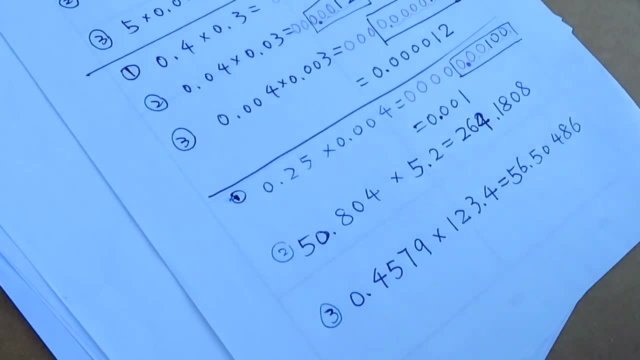 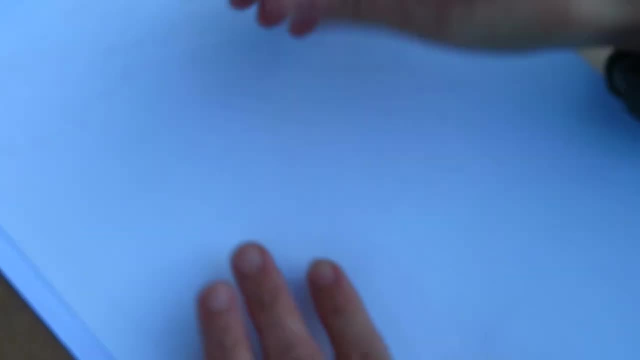 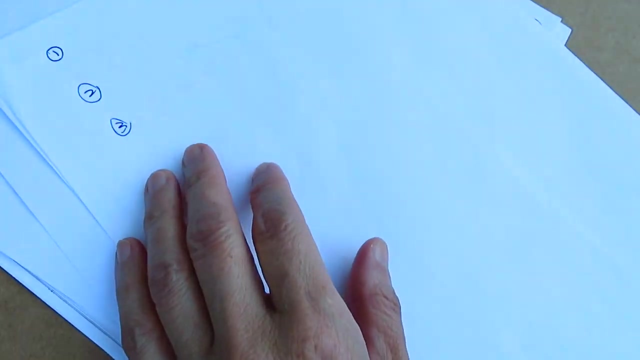 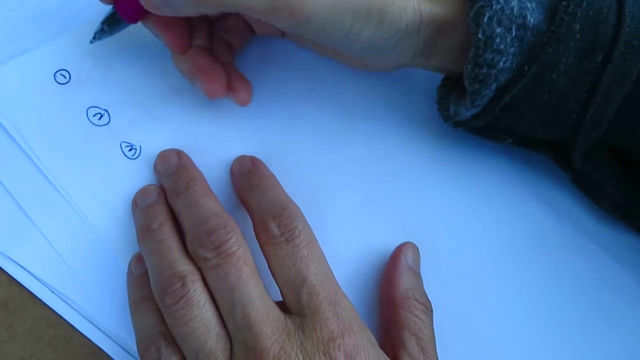 Okay, so we have done decimal multiplication of decimals. now we need to do some division of decimals. So first problem: we do some simple start from repetitive pattern, as we always do. So let's do a real number. it's an integer. 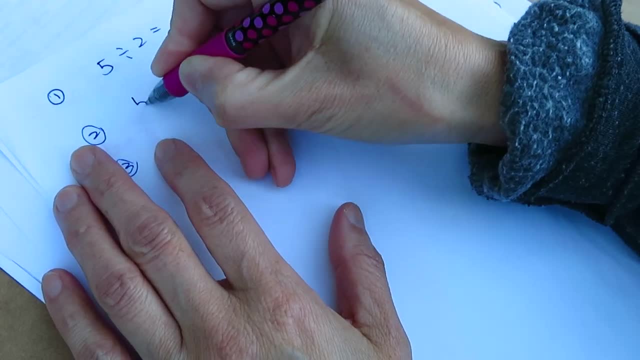 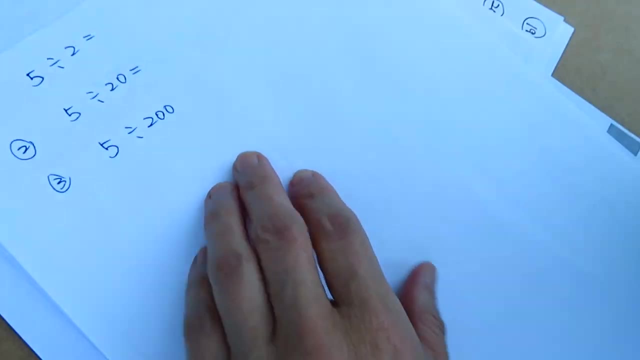 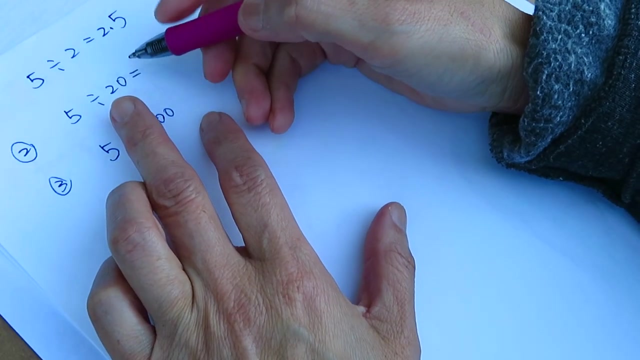 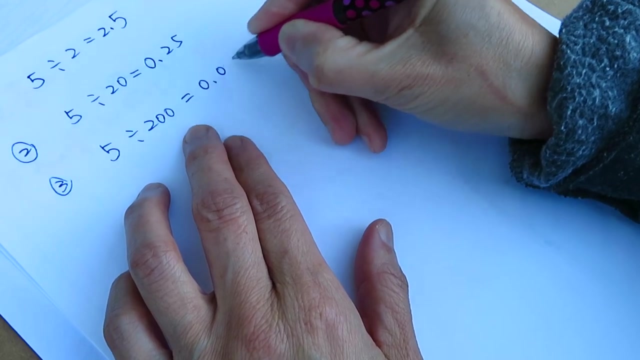 5 divided by 2,. 5 divided by 2, by 20,. 5 divided by 200.. So what do I do this? 5 divided by 2 is 2.5 and there is one zero, so 0.25, a decimal point. We need to move 1,. 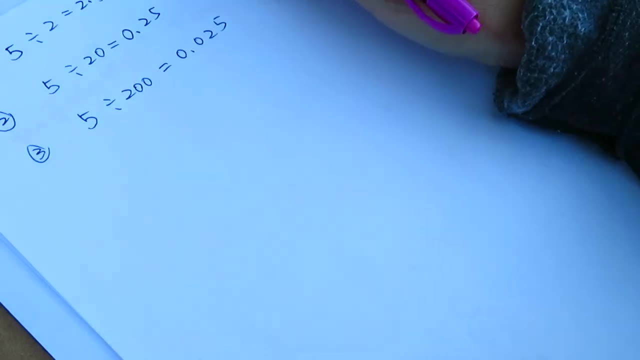 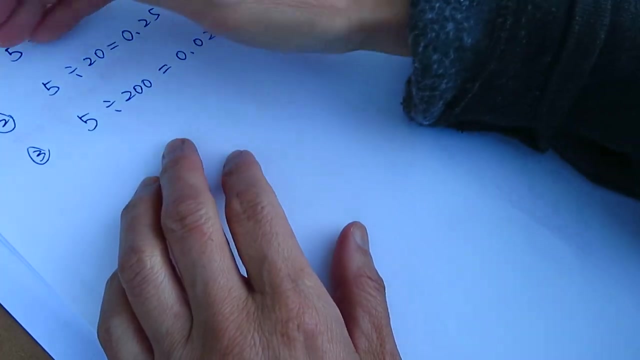 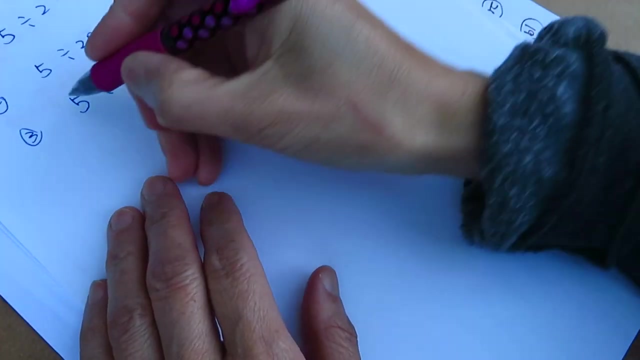 move 2.. but this does not this. if you do repetitively doing this, you can understand, but you do not have this base. it's kind of hard to understand or it's kind of kind of easy to get lost, right? okay, let's do this one now. first to this one five. 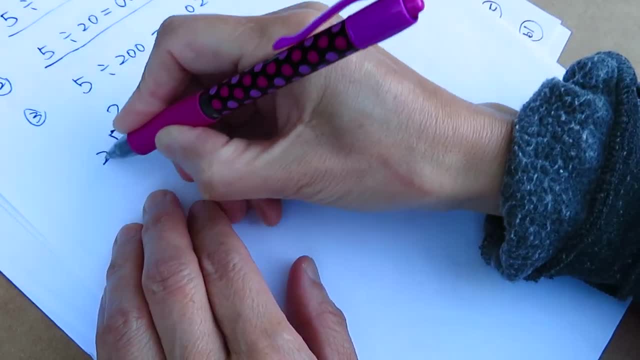 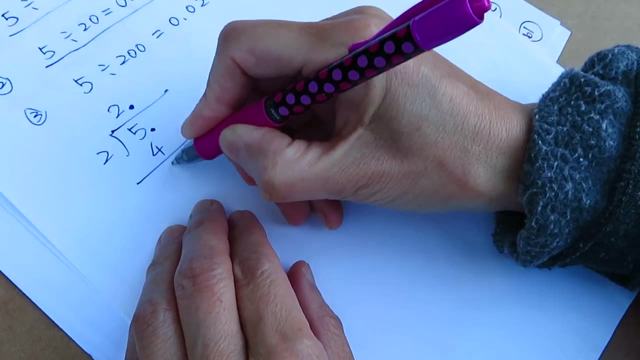 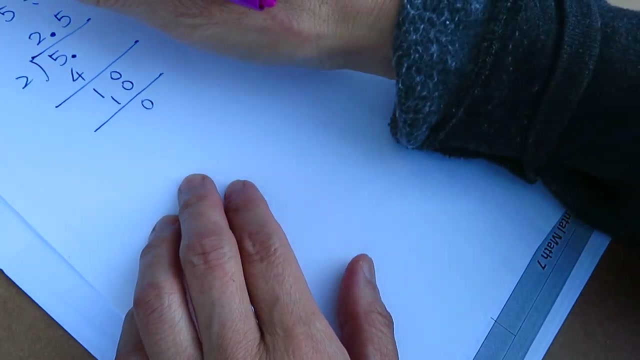 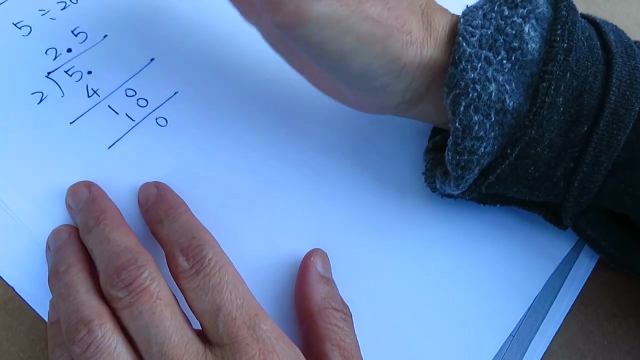 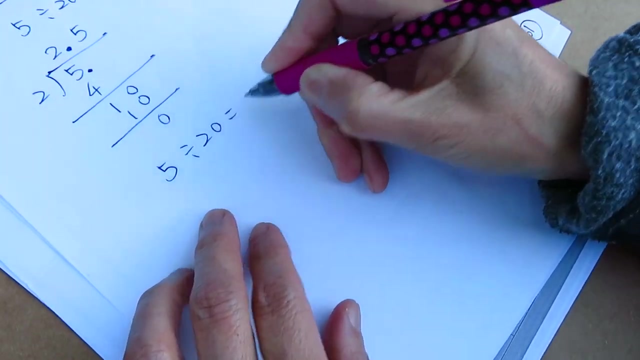 divided by two. two are 二得四. then put a decimal point here: 二五得十. so this is how I do. and five divided by twenty. it's whenever here with a zero I always have trouble. so when I do this, five divided by twenty, I move it one zero. 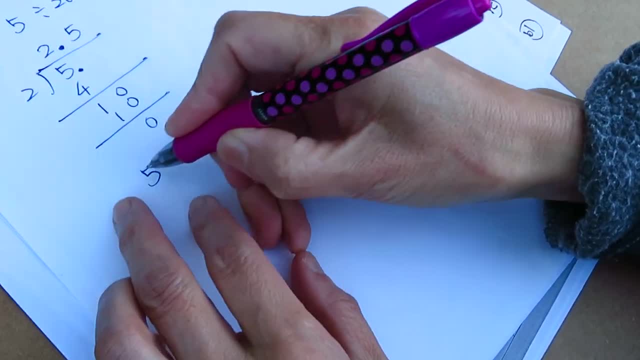 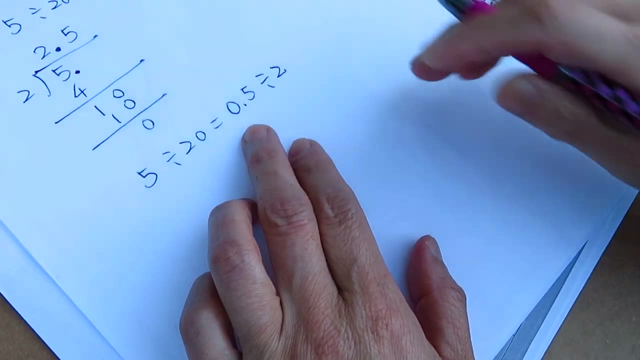 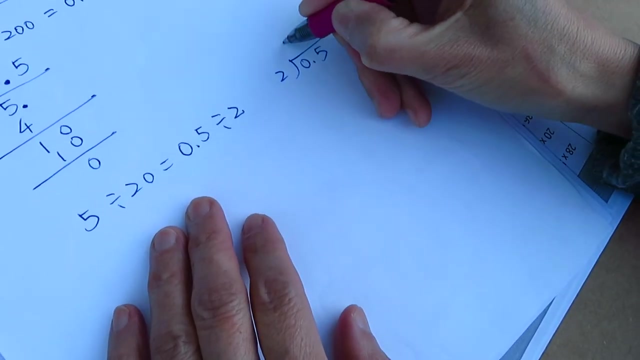 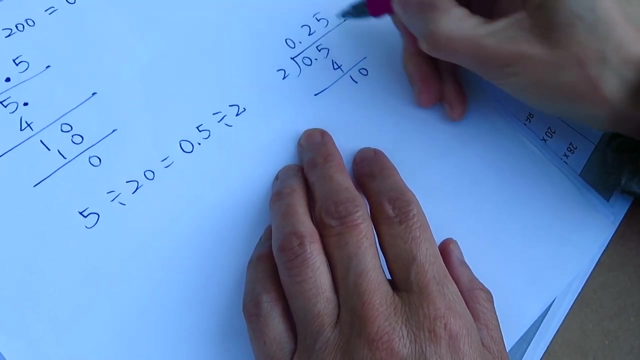 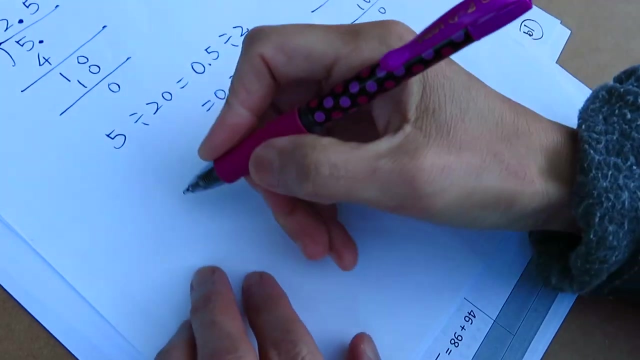 I cut out one decimal, oh, I cut out the zero and move decimal point here equal to zero point five divided by two. this is how I do. okay, zero point five divided by two. easy peasy. zero point 二二得四, so down. zero point two, five. I get it okay. two divided by five. divided by two. 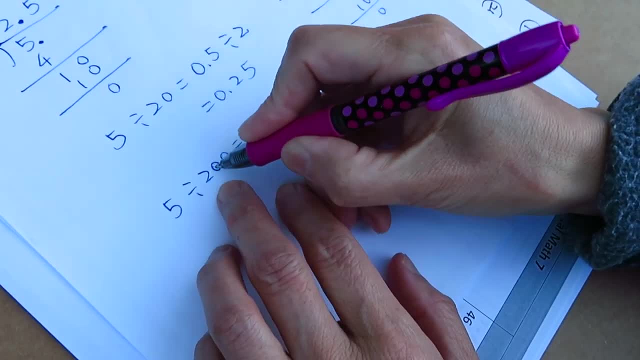 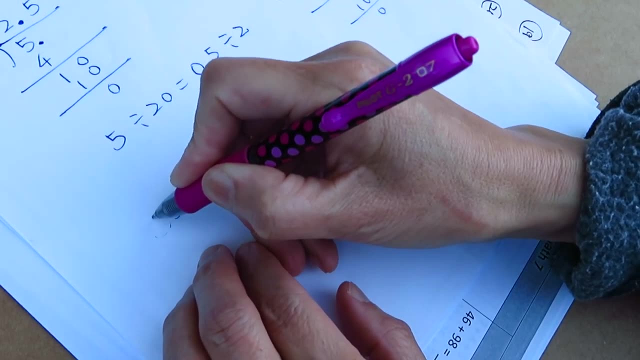 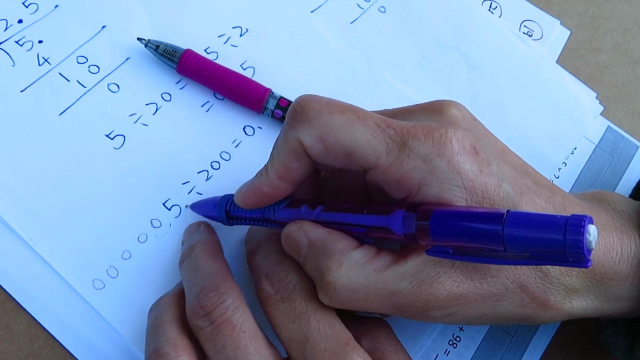 hundred. what do I do? zero point one, two, get out two points three, make a total of zero point four. okay, so I got three. okay, so two zeros and move decimal point one, two here. so same thing. i put a lot of zero in front and i need to exchange decimal point with these zeros. cut out two zero, one, two. 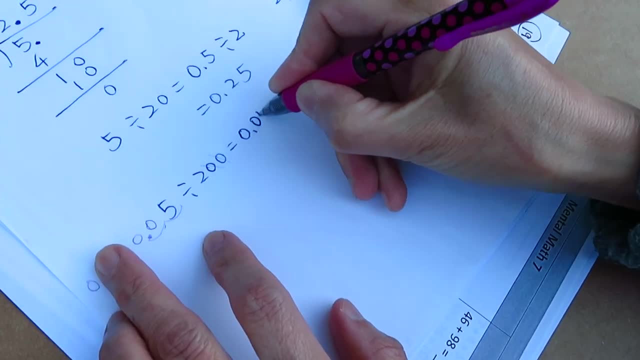 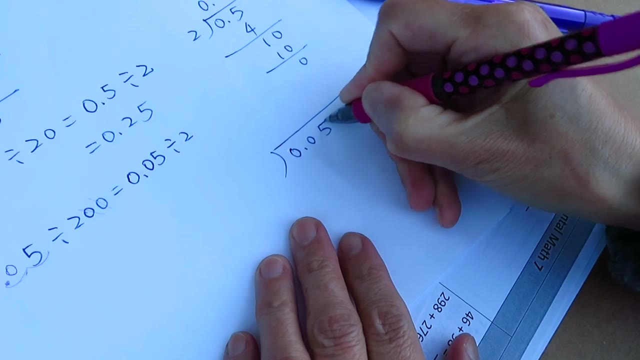 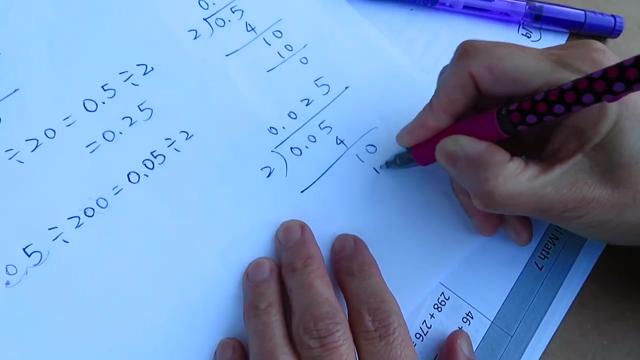 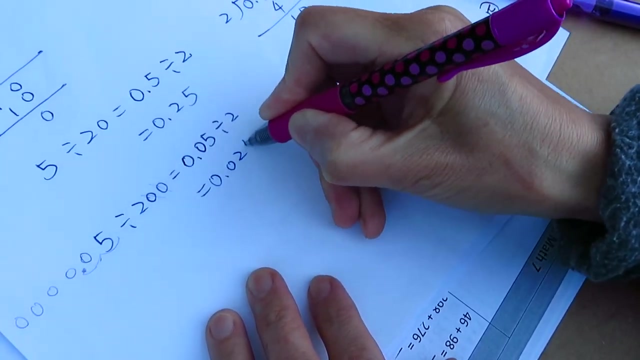 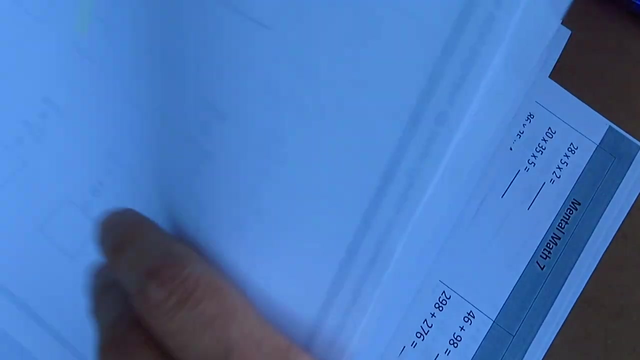 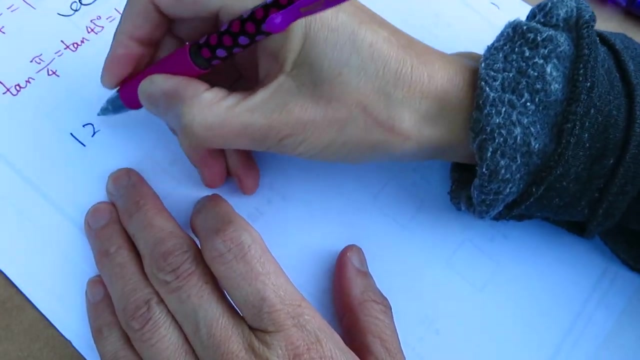 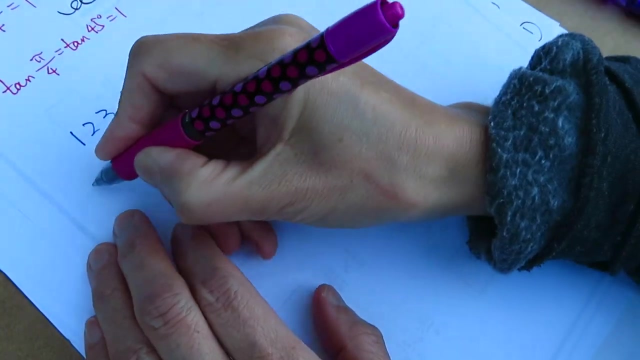 so zero point zero, five divided by two: okay. zero point zero, five divided by two: zero point zero, okay. so the result is 0.025. easy peasy, right now let's continue to do some bigger number, okay. so um, 123 divided by 300. what do we do? we change it into 1.23 divided by three. 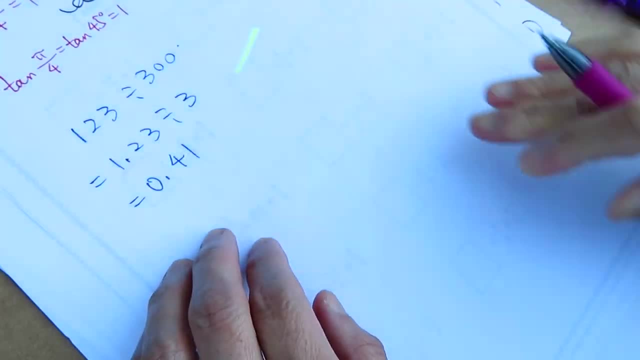 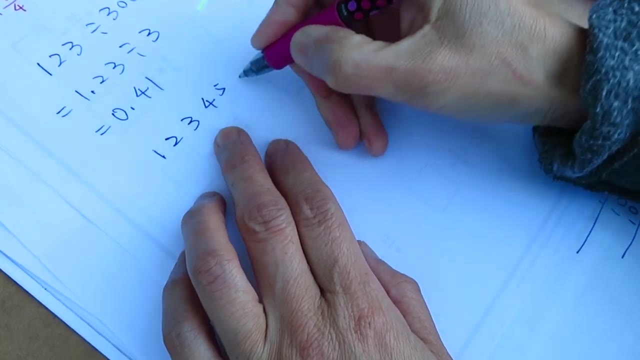 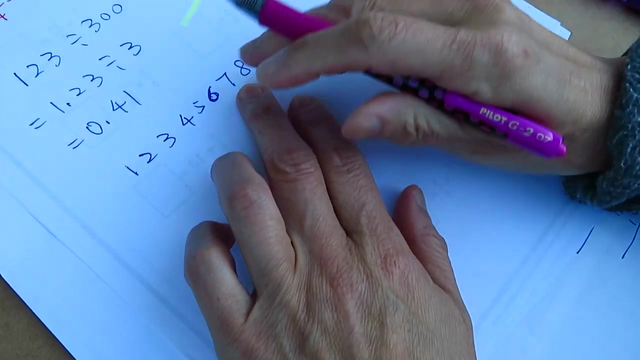 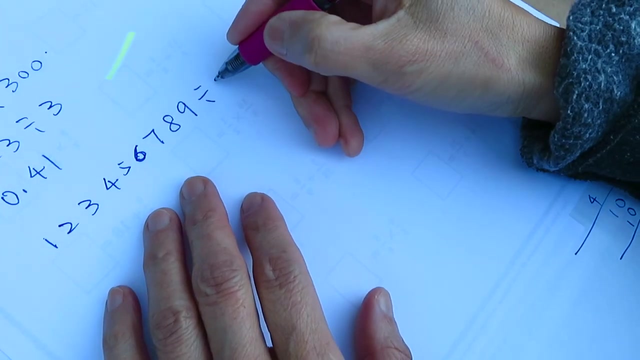 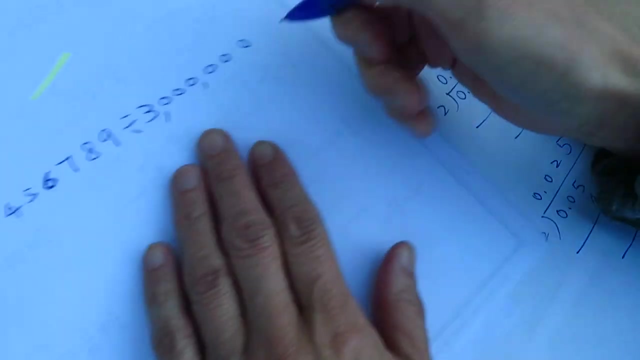 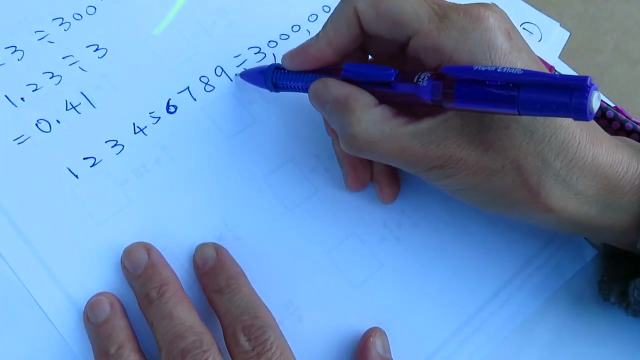 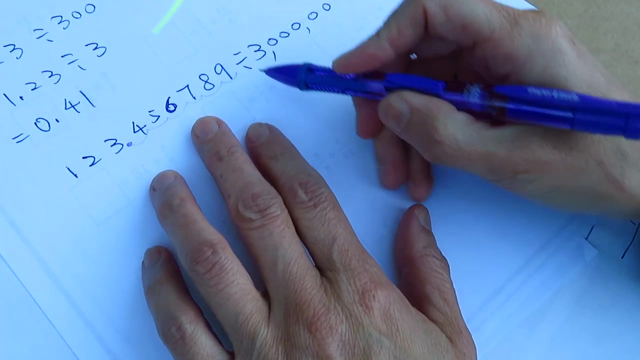 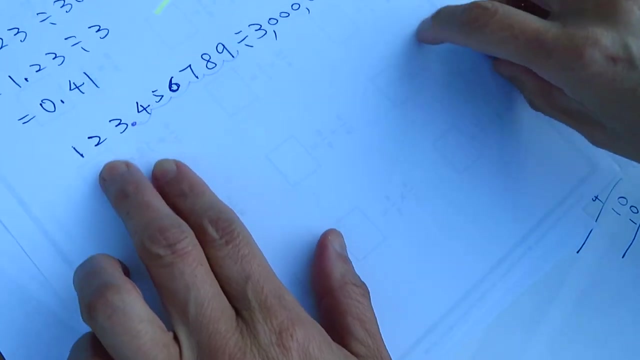 now it's easy: 0.41, right, okay. one, two, three, four, five, six, seven, eight nine, divided by, by um three million. okay, how many zero? we have one, two, three, four, five, six. okay, just move decimal point. one, two, three, four, five, six. again one, two, three, four, five, six. so one, two, three point four, five, six, seven, eight nine divided by. 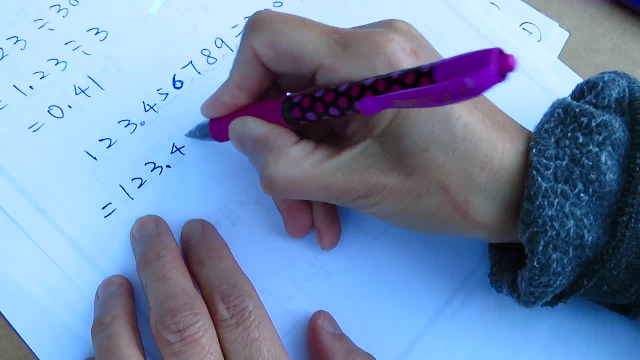 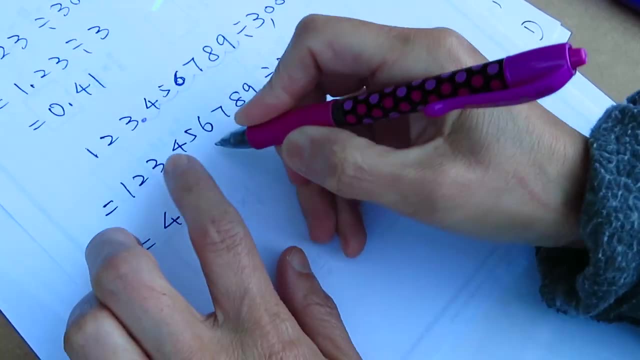 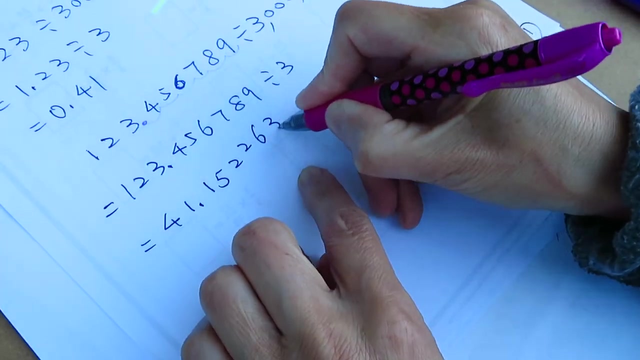 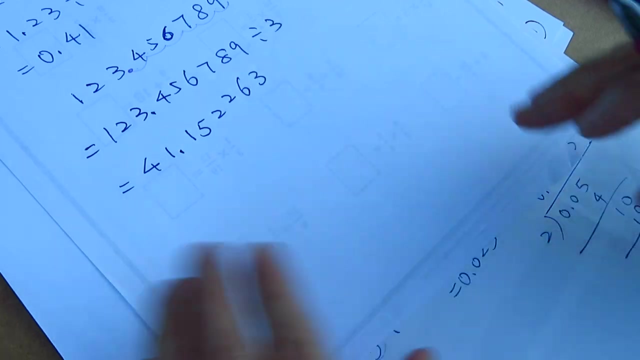 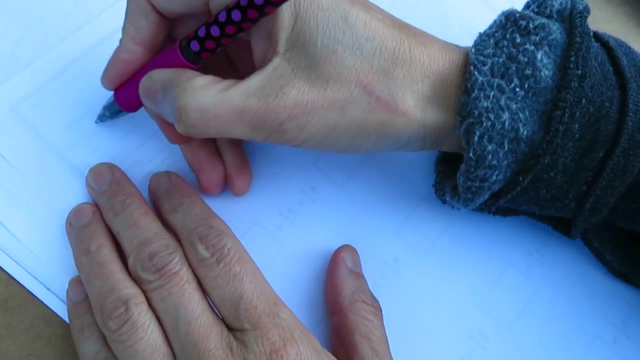 three, so equal to one. two, three point four, five, six, seven, eight, nine divided by three, equal zero or 2.04%. oh yi lands. please read both. this is the answer to everybody's question. so here is one zero, three. one in the il, the colonized view. no, get one in theEdisonese. OK. okay, now we do decimal divided by decimal. this one is 456.987.7: 1.256 individuals 25 years old. So this is the result that we get, okay. okay, now we do decimal divided by decimal. this one is 467.987.7.. 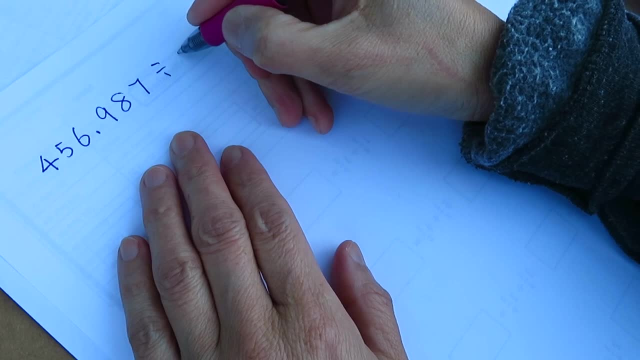 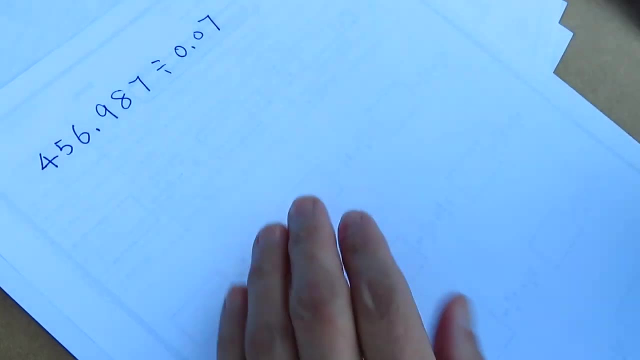 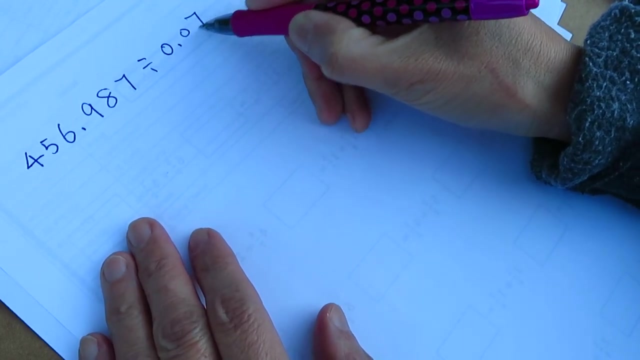 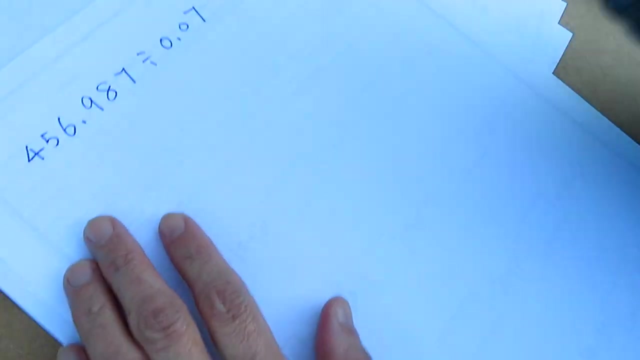 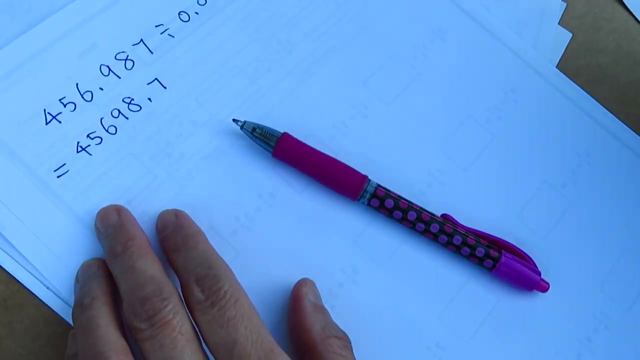 404. let's divide three by three steps: 0.07. let's say this one: okay, divided by the decimal, here that behind the decimal 2, so I need to get rid of this. divided by 007, I can change into 45698. divided by seven, because here I have two decimal. 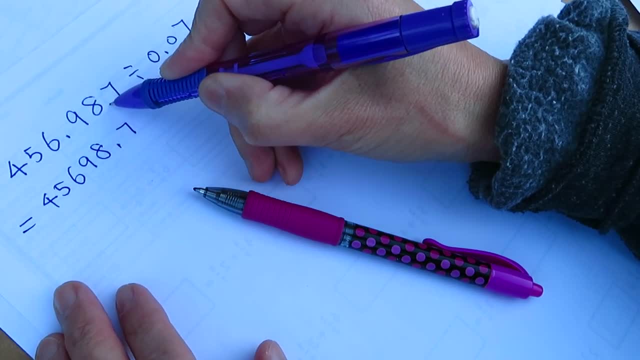 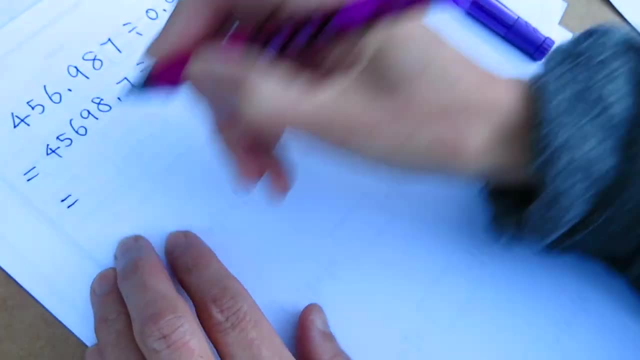 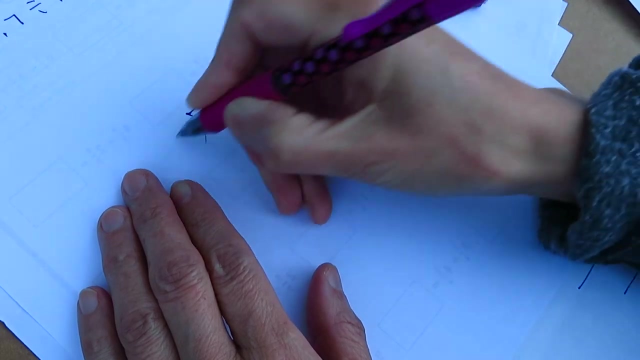 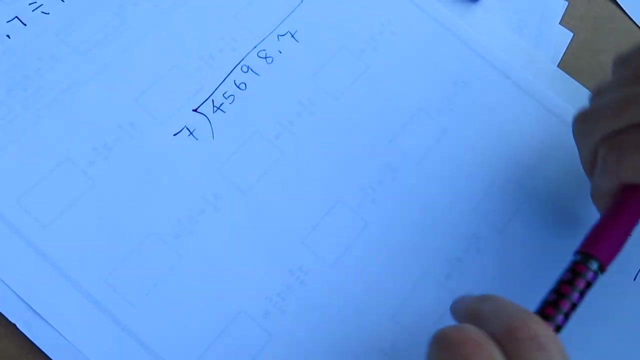 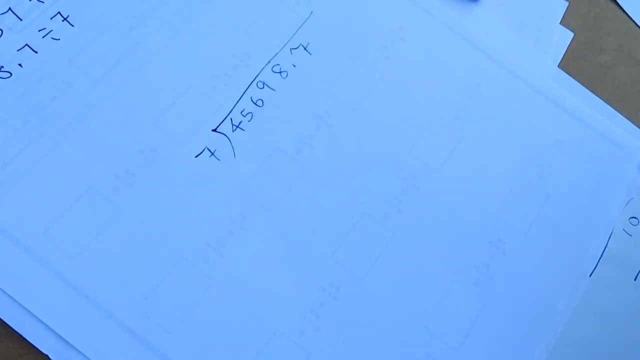 points I need to move the front. one, one, two, two, two change to here: divided by seven. equal four, five, six, nine, eight. point seven: divided by seven. okay, my pen is finishing up, I'm so happy. I just want to finish them. yes, almost, they're not it. 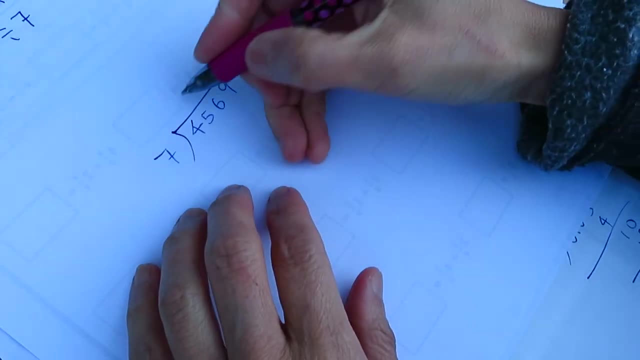 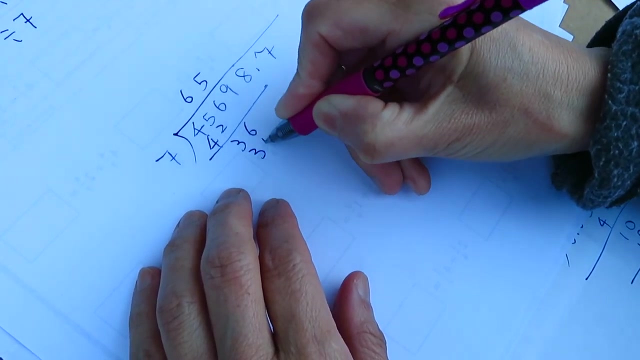 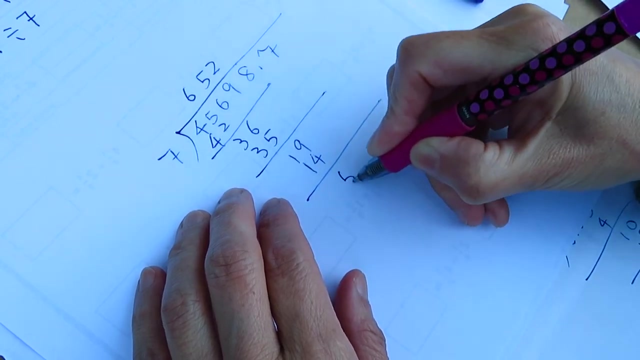 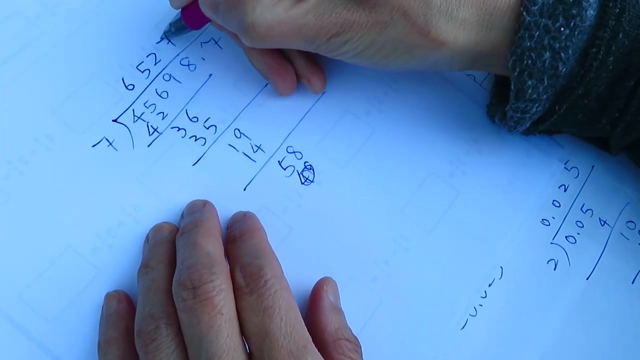 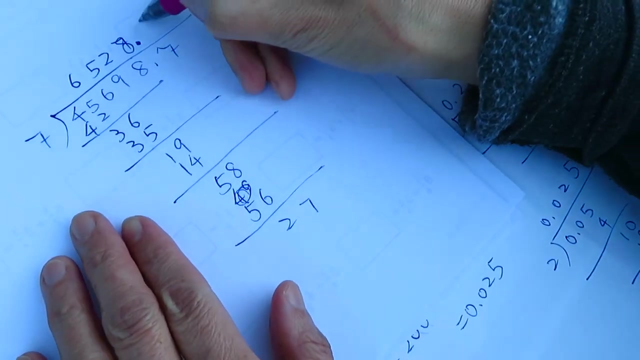 let me get it done. she knew she said she's our son. she knew who she says you're cool, she's you are she she. she said who's your bar she. she says she killed. oh no, she bought. she bought who. she knew I should. she sent she. and she knew we. 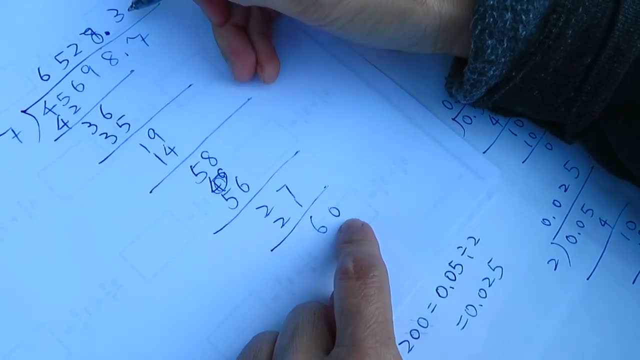 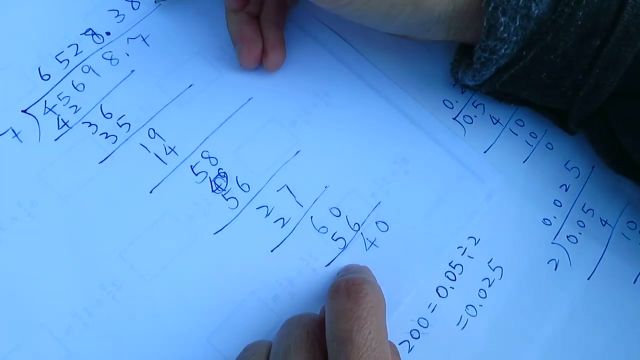 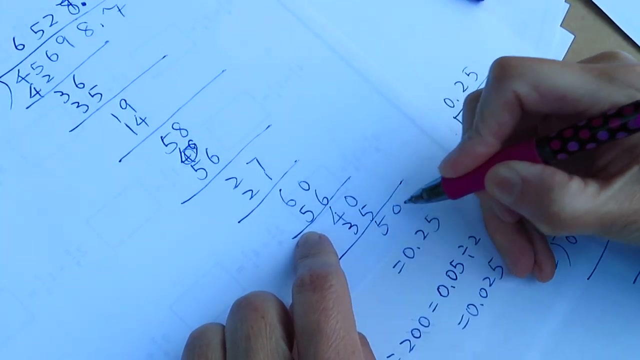 can do new. let's just keep on dividing new, new, new she she bought who should do so? she knows who she is and possibly would be able to tell you your brand name. you know you get your nonsense too. you got trouble. you got all the wrong bad. 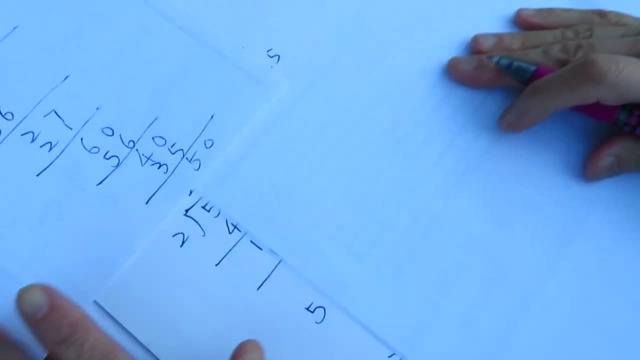 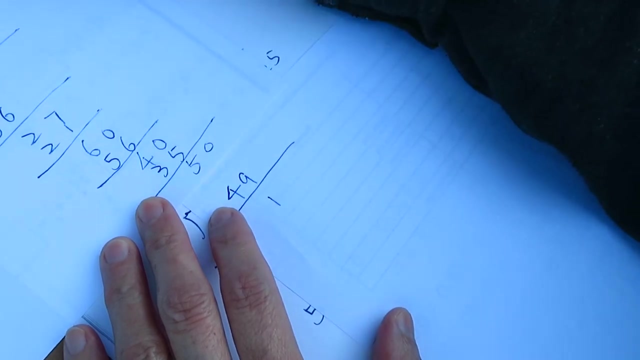 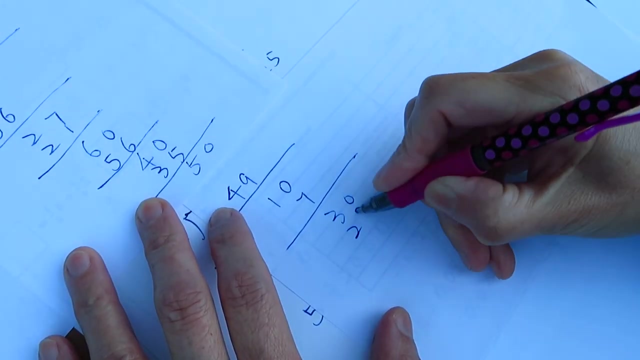 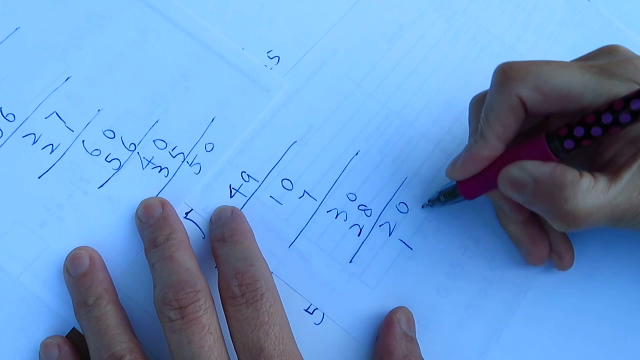 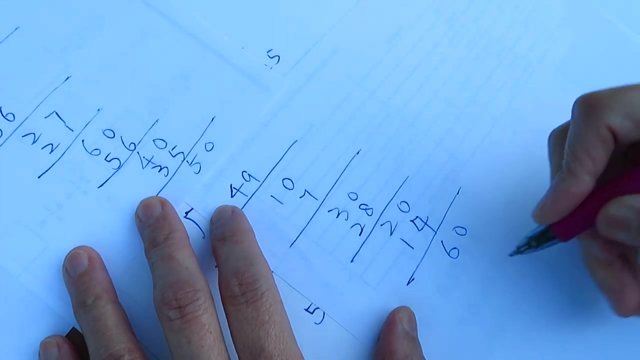 skin, you don't get all the wrong. 5, 3, 0, 0. what Finch ok. 0 G, 7, 28,, 2.. 2, 7, 1, 14,, 60,, 7,, 8,, 50,, 6,, 40. 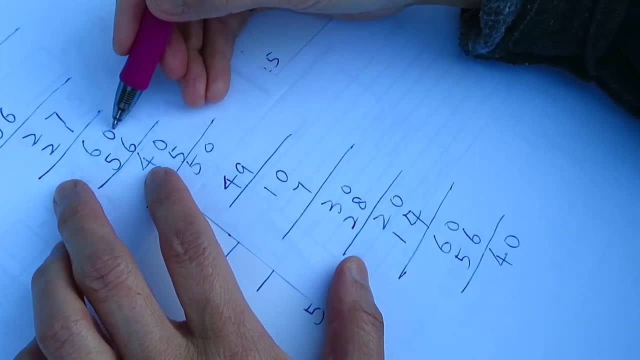 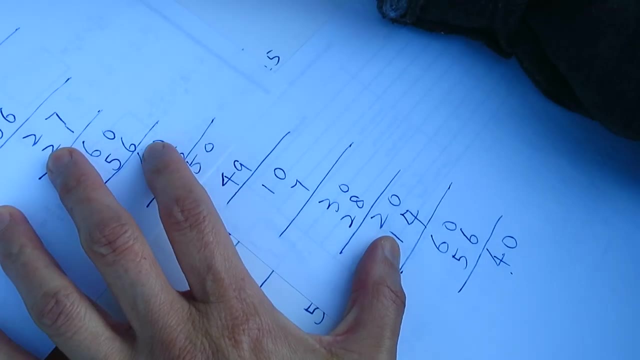 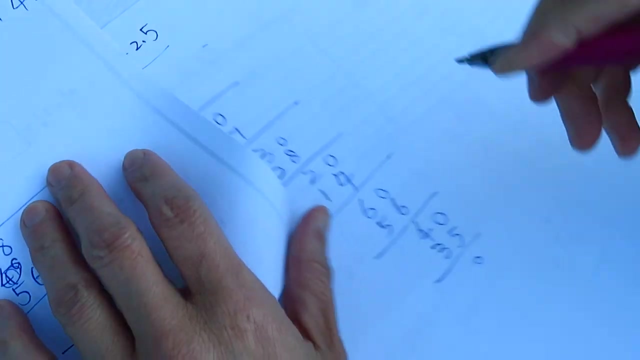 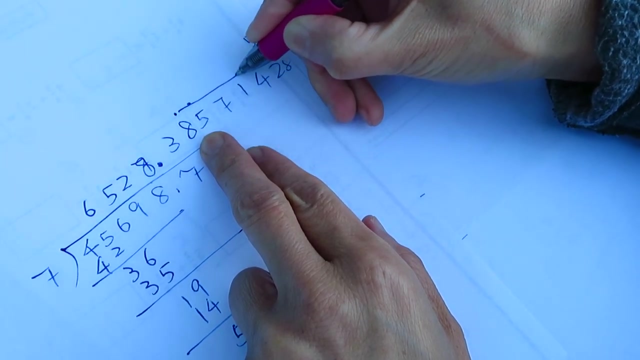 Oh, 4,. we are repeating Now 4, 8, and then 5, 8.. 5, 7, 35,, so 8, 5.. So here is the repeating: 8, 5, until here. 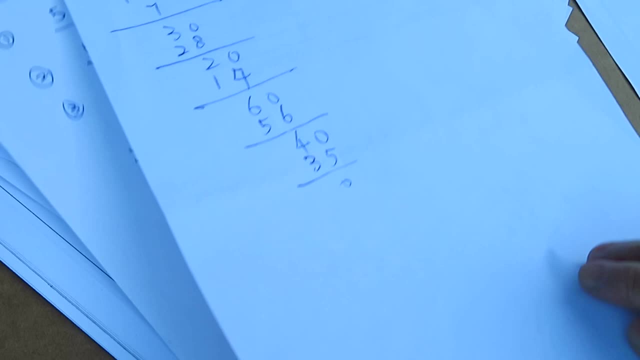 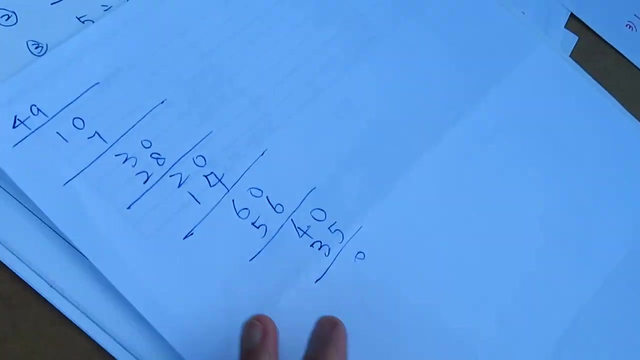 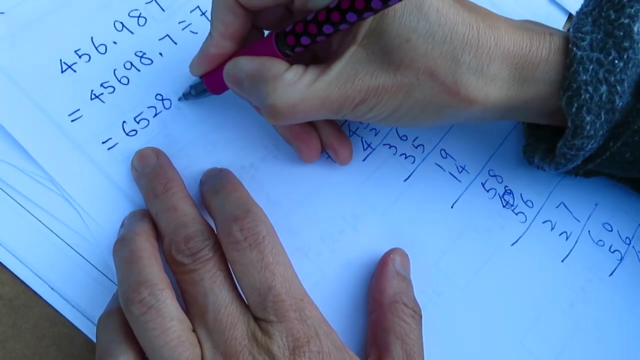 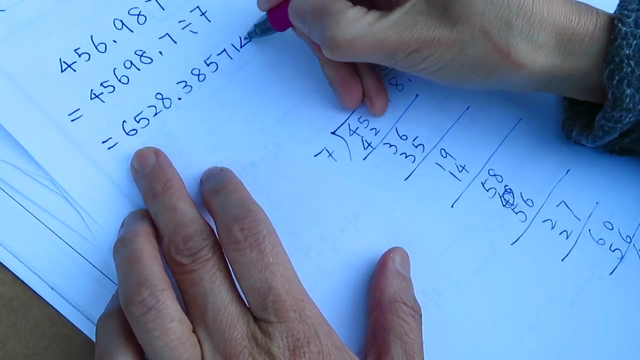 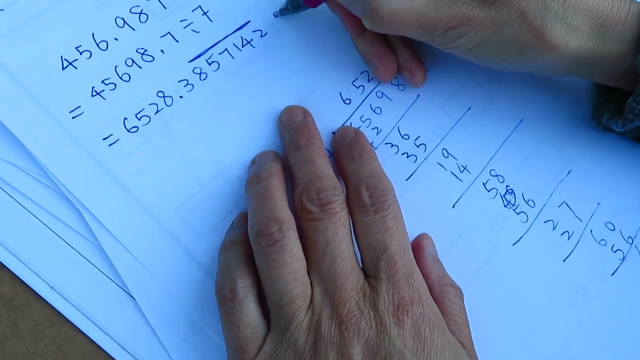 So our result will be: where is our number? Okay, so 6.. 6, 528.3,, 8,, 5,, 7,, 1,, 4,, 2.. And here is the repeating, And then keep on. 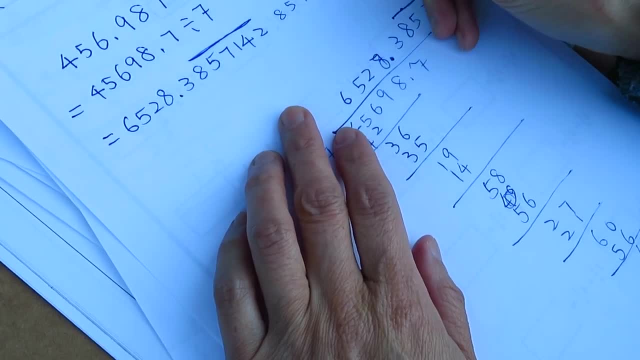 8, 5, 7,, 1,, 4, 2.. 8, 5, 7,, 1,, 4, 2.. 8, 5, 7, 1,, 4, 2.. 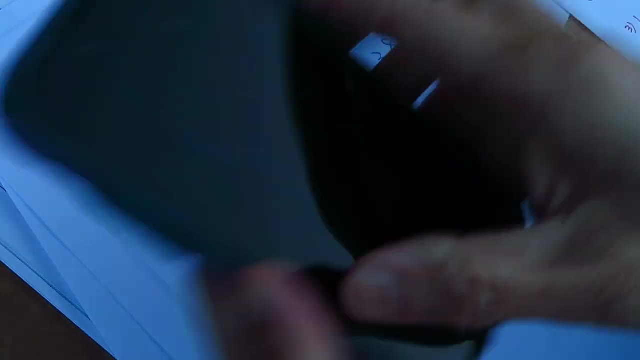 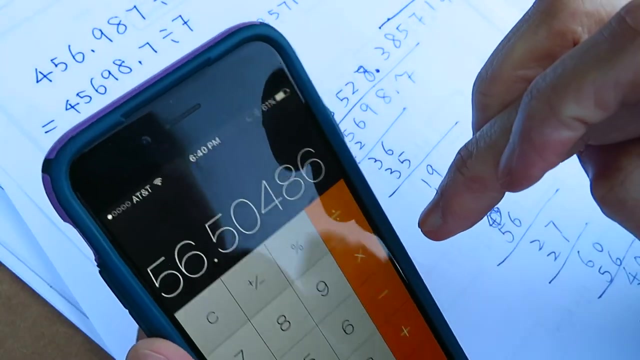 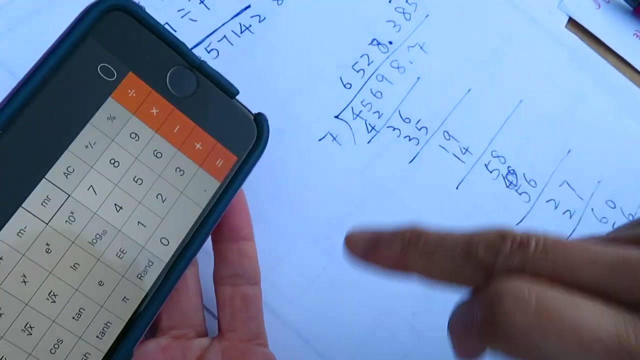 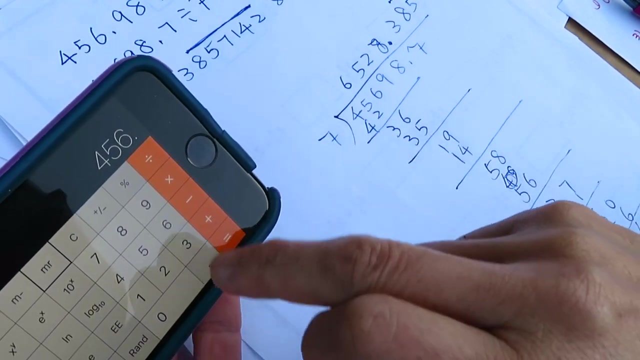 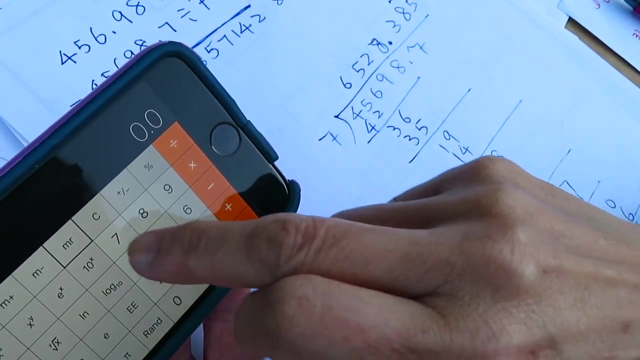 This is the repeating. Okay, let's see if we have done a right, good job in this. Well, this is a little bit too long. Let's see, Turn it around. Turn it around: 4, 5, 6.987 divided by 0.0.. 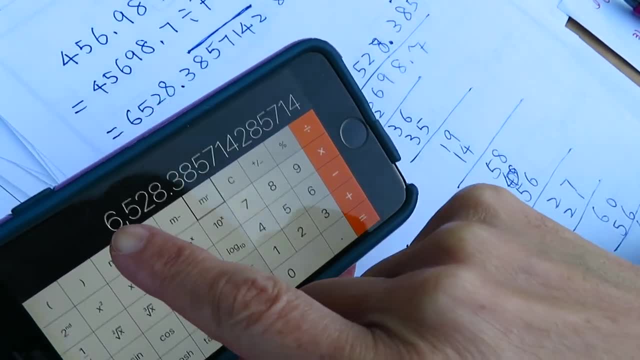 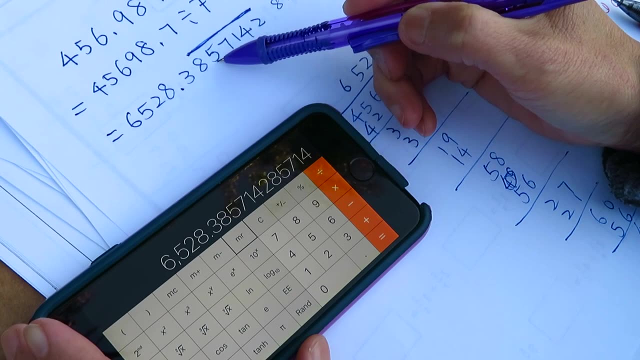 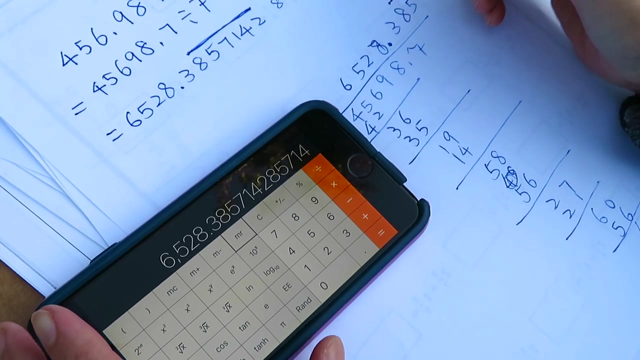 7, 8,, 5, 5.. 6, 528.38571,4,. 2, 8, 5, 7, 1, 4, 2, we yes, Yeah, yeah, yes. 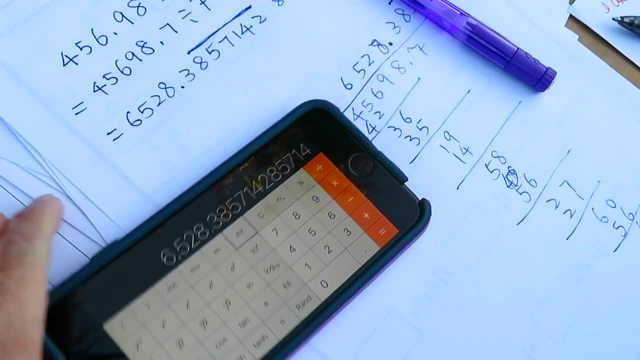 Yes, yeah, yeah, yes, I made it right and I'm so happy. Yeah, Yeah, the joy of큒. Yeah, I'm so happy, right, I'm so happy right. Yeah, Right, Yeah, Yeah, Yeah.